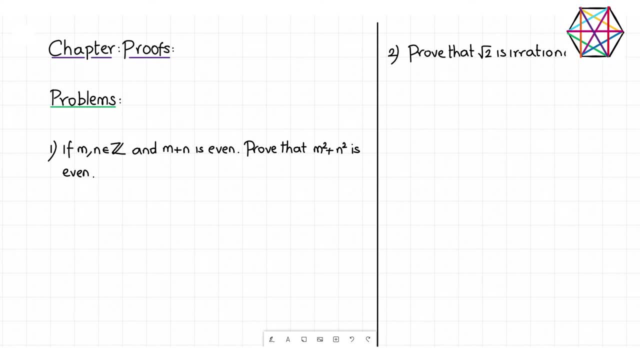 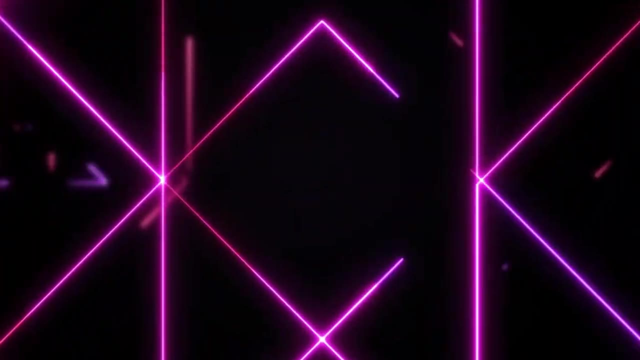 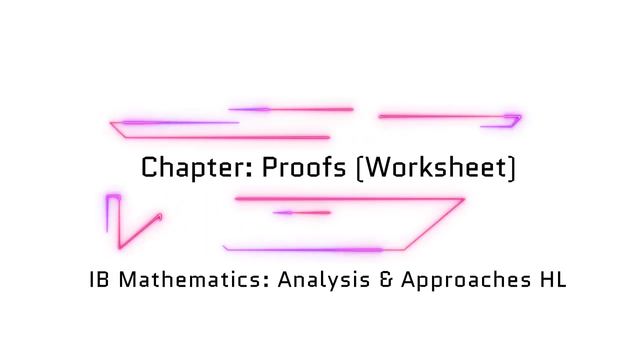 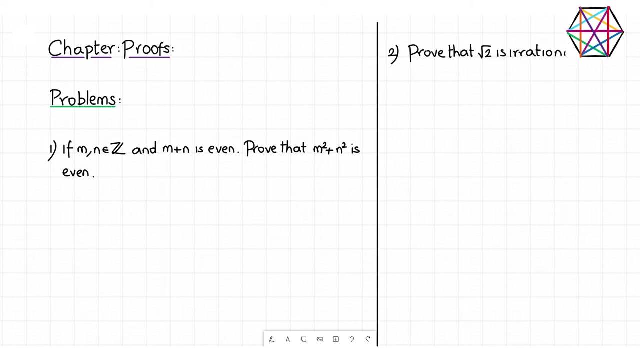 Hi everyone. In this video lesson we are going to discuss problems from the chapter Proves, which is one of the chapters in higher level mathematics: analysis and approaches for the IB Diploma. We are discussing problems from the chapter Proves and we have few different types of 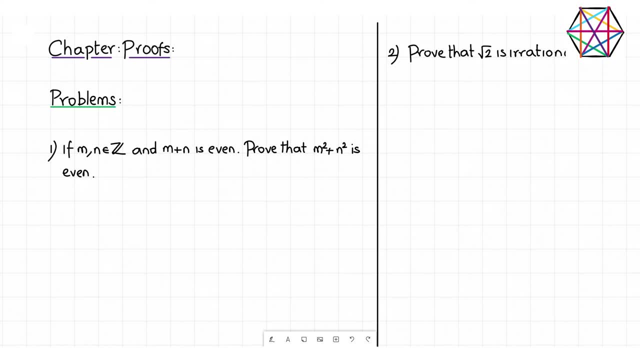 proofs. What are they? We have direct proof. We have proof by contradiction. It comes under indirect proof. Proof by contradiction comes under indirect proof And we have proof by contrapositive. And we have proof by exhaustion. We have proof by mathematical induction. These are different ways of proving a result or a theorem in mathematics. 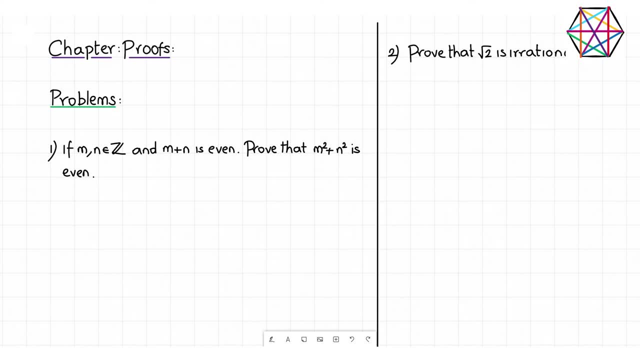 And there is no rule as to which type of proof we need to use in which situation, in which problem or theorem. There is no rule, nothing for that. It comes only with practice. And also there are problems. there are theorems where we can use multiple proofs, multiple. 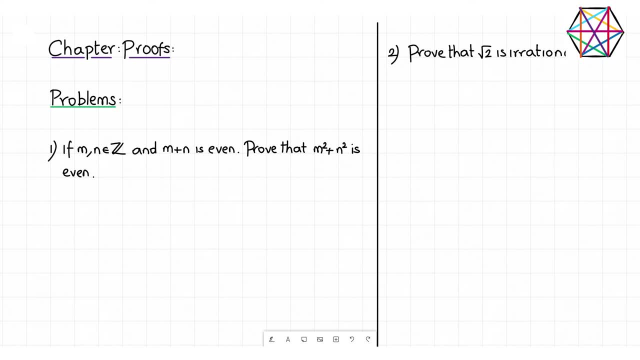 types of proofs For the same result. you can use proof by contradiction or you can use direct proof, And sometimes both will be even equally good. Even that is possible. That's a rare scenario, though. So when we are solving problems, you will get better. 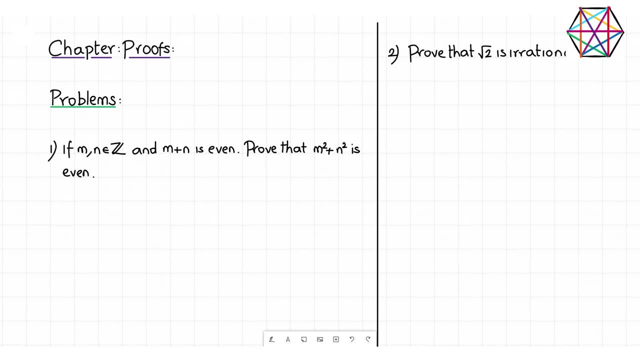 idea about all these different types of proofs. I tried to cover almost every type of proof in today's class, So yeah, So starting with problem number one. Problem number one: if m and n are integers, both m and n belongs to set of all integers. 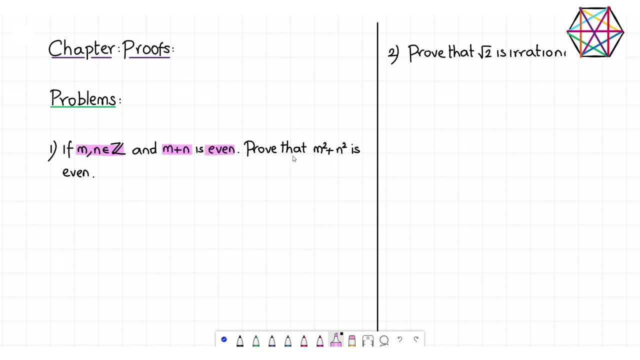 and m plus n is even, Then prove that m squared plus n squared is also even right. m and n, both of them are integers, And it is also given that m plus n is an even number. Based on this, we need to prove that m squared plus n squared is, And here you have to prove that. 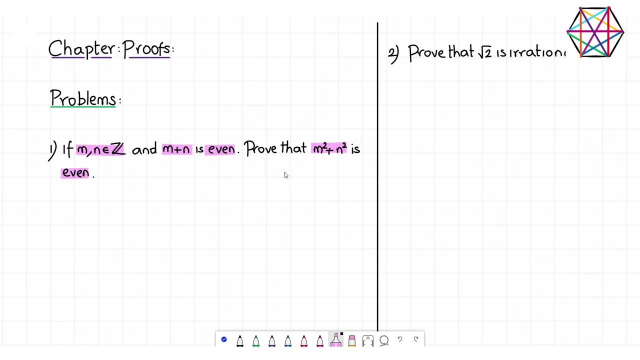 m squared plus n squared is an even number. And if m plus n is an even number, then proof square is an even number, right, okay? so how to prove this? check this. so consider m and n. both of them are integers and m plus n is even, it's given. consider the given statement. 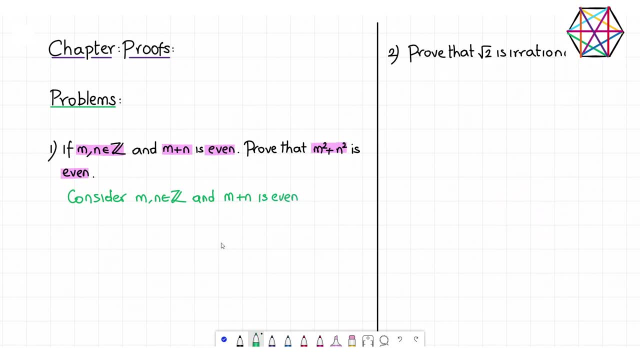 this is given. now, since m plus n- both of them are m plus n- is even, it implies that m and n, both of them are even, or m and n, both of them are odd. agree. if sum of two numbers is even, if sum of two numbers is even, then we have only two possibilities. what are they? m and n, both are even. 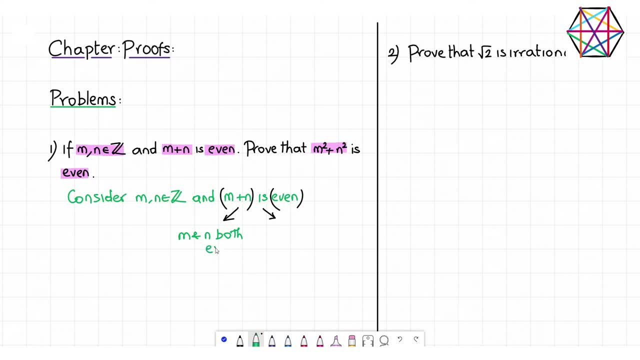 yes or no, they both are even. or m and n. m and n, both are even, both are odd. does it make sense? you didn't know this? okay, simple listen. you take any two odd numbers, three and seven, add them, you get even number. it requires a formal proof. this by itself, you know. 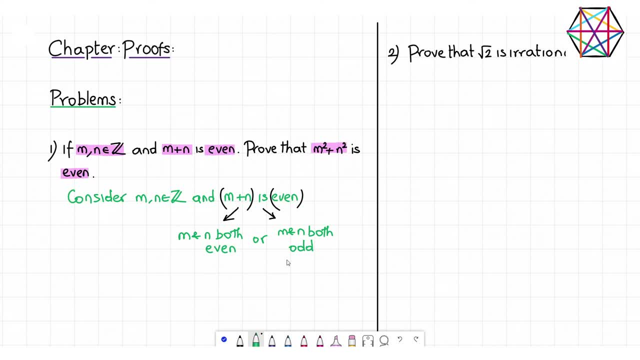 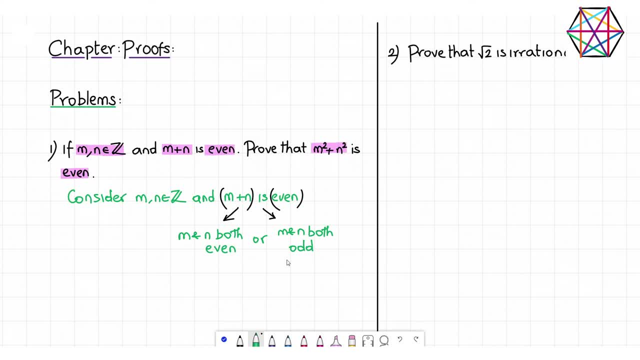 you know it's a statement that requires formal proof, but let's not get into it. it's like a: take any two odd numbers, take 13 and 15, add them, you get even number. right, you get 28. you take any two even numbers: you add them, you still get an even number. you take any two even numbers, add them you. 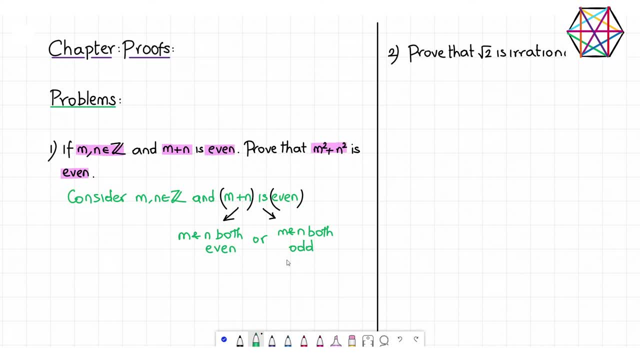 still do get an even number. did you get this? but when you take one even number and one odd number, in whichever order- odd plus even or even plus odd, doesn't matter, you will get odd number, yes or no. what is uh four, which is even number, plus uh 11, which is odd number? what is even plus odd? 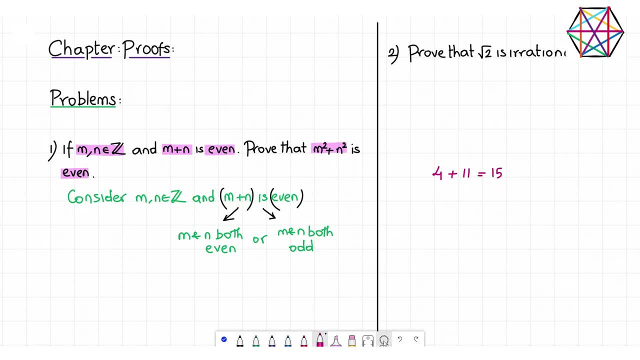 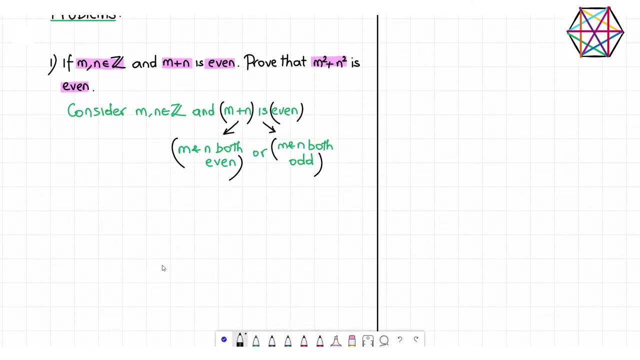 it's odd number. did you get this? so it's given that m plus n is even. so we know that there are only two possibilities. okay, only two possibilities: both m and n are even, or both m and n are odd. yeah, okay, so now how to proceed from there? check this case one. 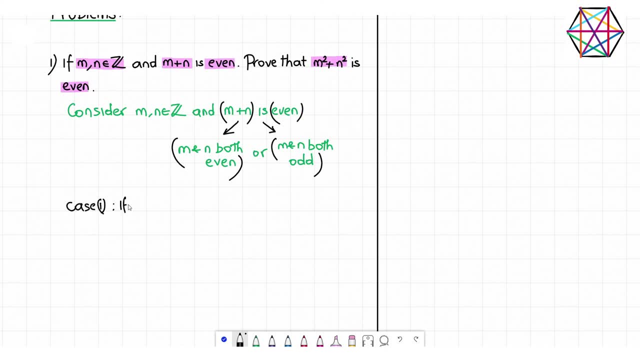 if m and n both are, even if m and n both are even, what can you say now? if m and n both are, both are, even if m is even. don't you see? m square is even yes or no. what is the meaning of? what is the meaning of m square? 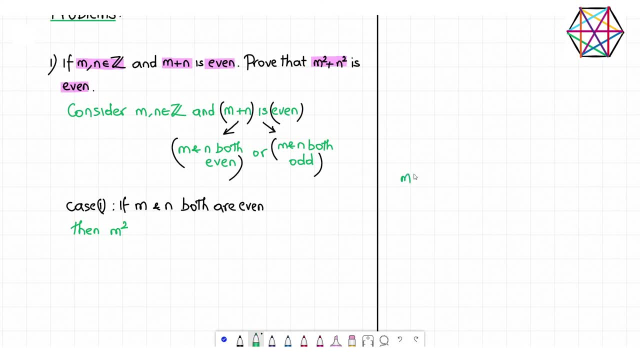 you're multiplying this number m by itself. yeah, what's the meaning of m square? it is m multiplied by itself, right? so what is even number multiplied by itself? how is it even? okay, what is? what is? what is the definition of even? what is the definition of even? 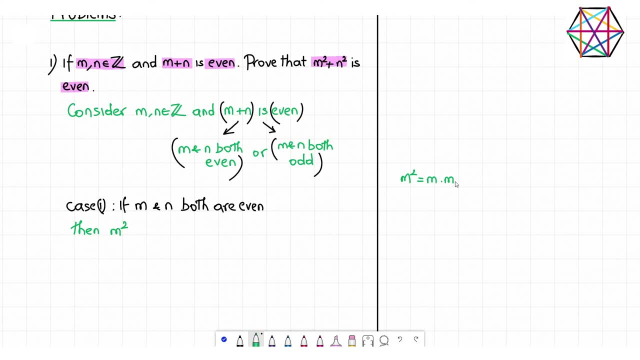 multiple of two. okay, yeah, so i just said m is even so m by itself is a multiple of two, and that you're multiplying by another multiple of two, so it's guaranteed to be a multiple of two. you see, in fact, when you multiply even number by any random integer, not necessarily even number. 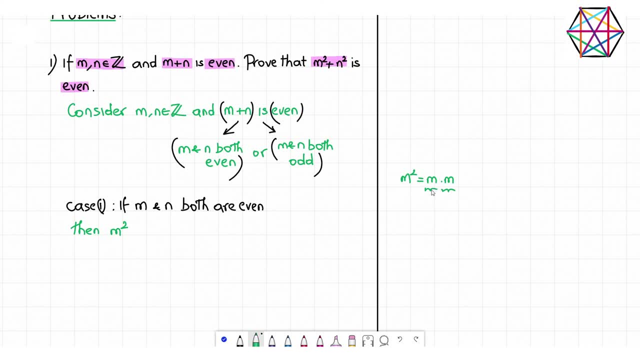 even if it is multiplied by odd number, it is going to be even. does it make sense? no, you take any random odd number, okay, 17. but when i multiply it by even number, say 8, the result will be even guaranteed, because 8 by itself is a multiple of 2, right? 8 is a multiple of 2 and. 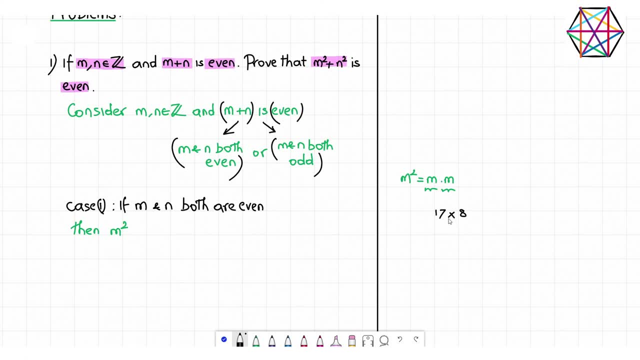 on top of that, i'm multiplying some other number. i don't care what that number is, even or doesn't matter. ultimately it's going to be a multiple of two. therefore it's even. yeah, got it okay. so now, since m is even m square, is even right. and since n is even n square, is what even right? so thanks. 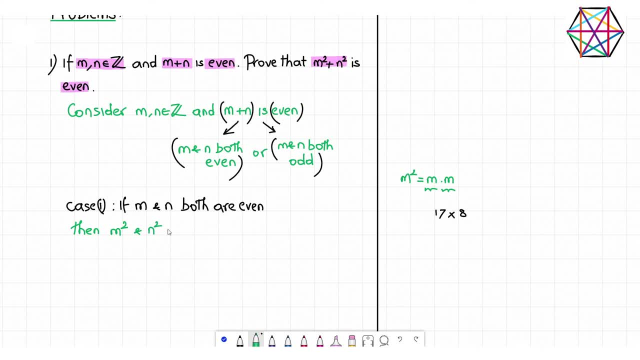 what even right then, m square and n square. both are even: m square and n square, both are even. now, if these two numbers are even, what can you say about their sum? just a while ago i explained if these two numbers are even. these two numbers are even. yeah, so m square plus n square is even. 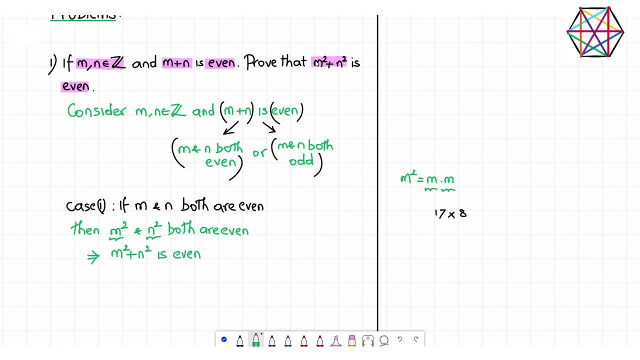 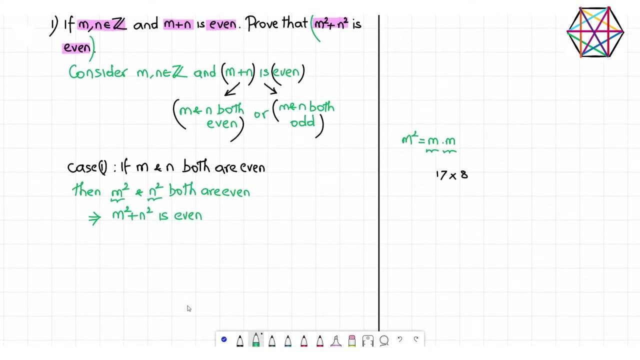 so this is exactly what we are asked to prove, right. prove that m square plus n square is even. but we're not done though, right, there is another part to it, there is another. we discussed only one case. now we have to discuss the other case, right? what is the other case? 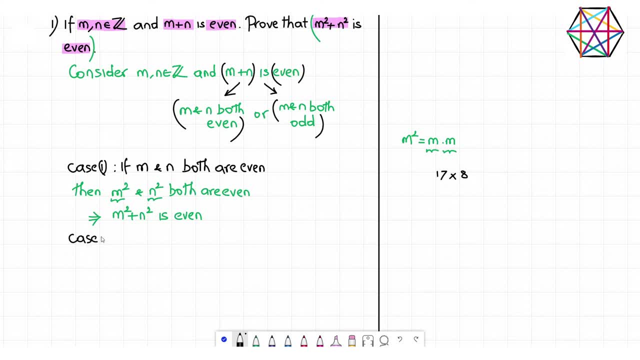 yeah, the other case is m and n, both are, or both m and n are, or okay. so how to? how to proceed here? if m is odd number, m is odd number, then what can you say about m square? easy guess: odd. do you see why? look at this equation once again. m square means m times n. right now you? 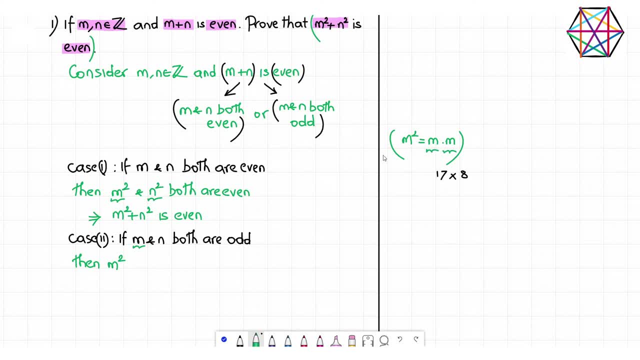 know that m is a odd number. odd number is any number, any natural number which is not a multiple of two. odd number is, or you can even say, integer. odd number is any integer which is not a multiple of two. so this is not a multiple of two, not this one is a multiple of two. it's of course. 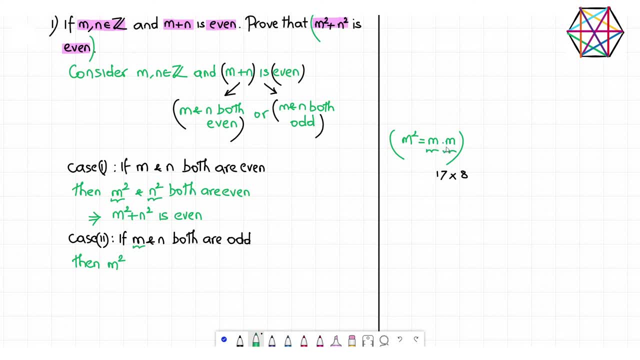 the same number, right? so neither of them is a multiple of two. so when you multiply them, of course you won't get a multiple two, right? that's it. so if m is odd, then m squared is odd. same logic applies for n. since n is odd, we know that n squared is odd. so 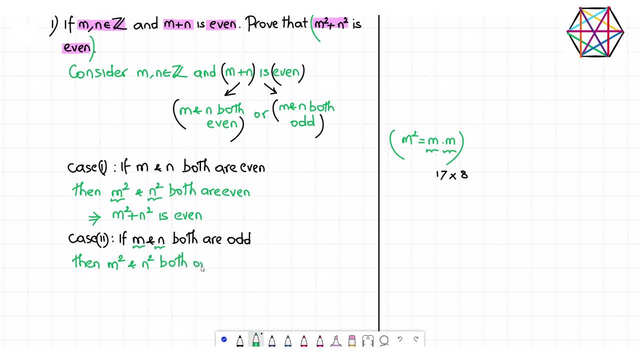 So the conclusion is: both m square and n square are odd numbers. This implies: now tell me what is sum of two odd numbers. Yeah, this is odd. this is odd. What can you say about sum of two odd numbers? It is even. 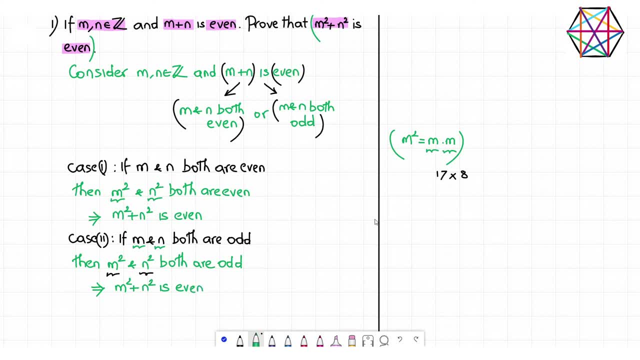 Did you get this? You take any two odd numbers, add them, we get even. That is something I have explained just a while ago. No, no, no, I said when both are even, the sum is also even, not odd even. 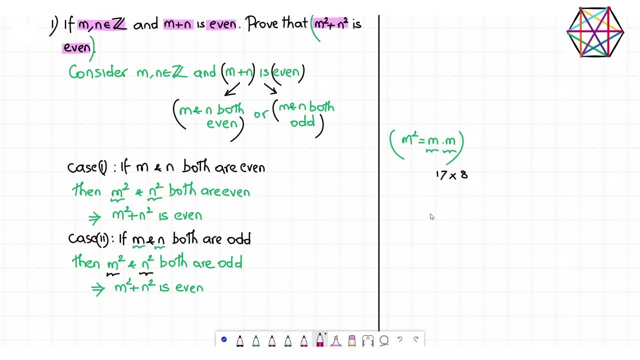 Yes, yeah, we can certainly do it. okay, You have two numbers. okay, say m and n. I am not talking about m and n from this problem. okay, some random integers: m and n. So this is a multiple of two. 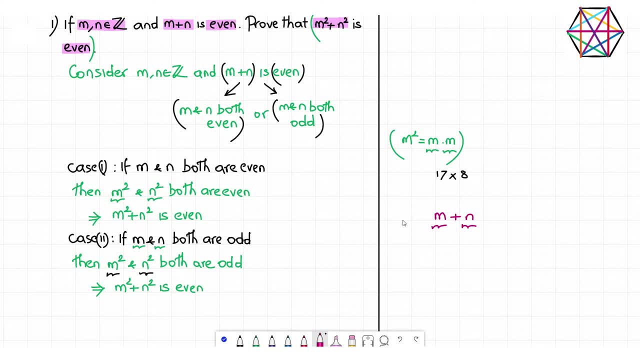 And this is also another multiple of two. When you add any two multiples of two, what do you get? Multiple of two. any questions about it? So it proves that it is even right. But when it comes to odd, listen, when it comes to odd, if m is odd number, then m can be written as 2p plus 1.. 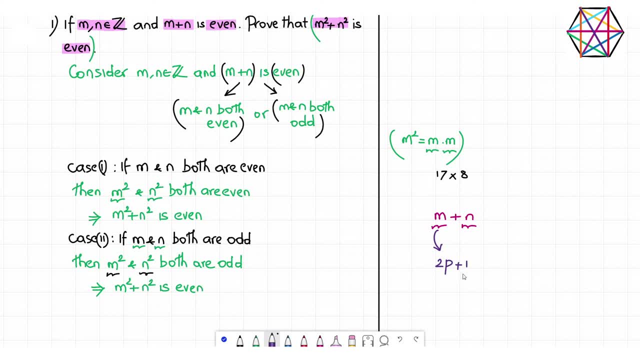 What is the meaning of it? What is the meaning of it? This odd number must be the next number of some even number. Yes or no? Every odd number is the successor of some even number. Okay, so this odd number m is successor of some even number, right? 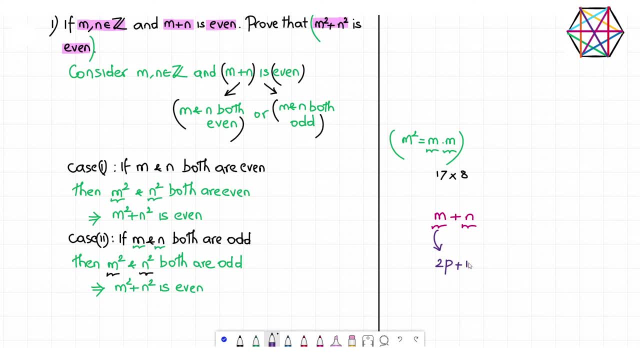 So it is 2p. 2p means what? It is? some even number plus 1.. Yeah, Yeah, you can write it like 2q plus 1. Then you can add them. you get 2p plus 2q. 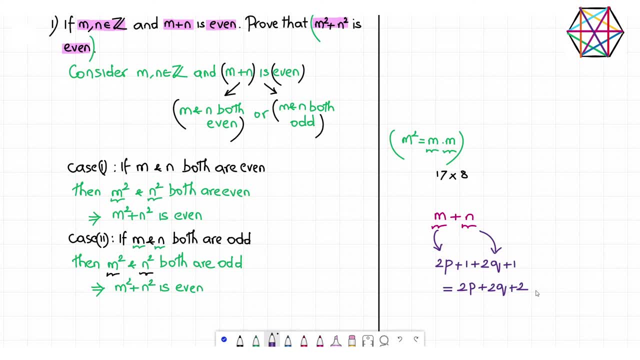 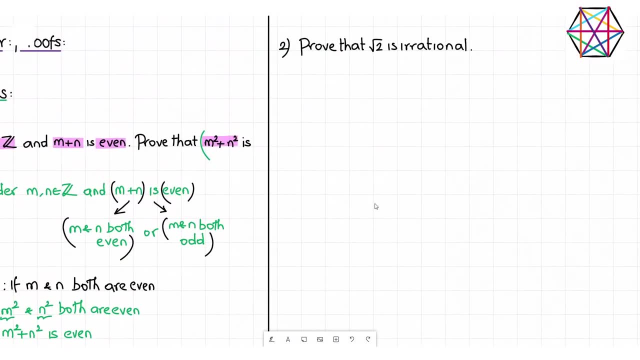 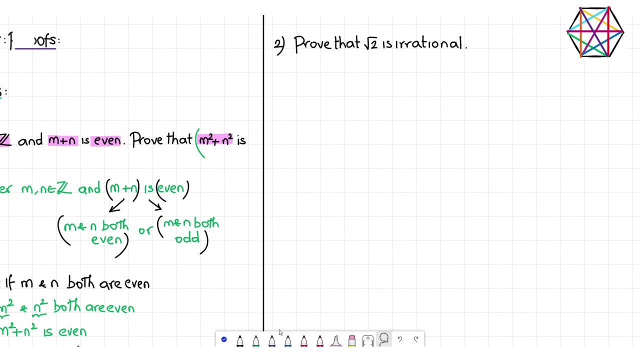 2p plus 1q plus 2.. Everything is even, So the sum is again even. Did you get this? Problem number 2.. This is a classic problem, Problem number 2.. Check this. What is the problem here? 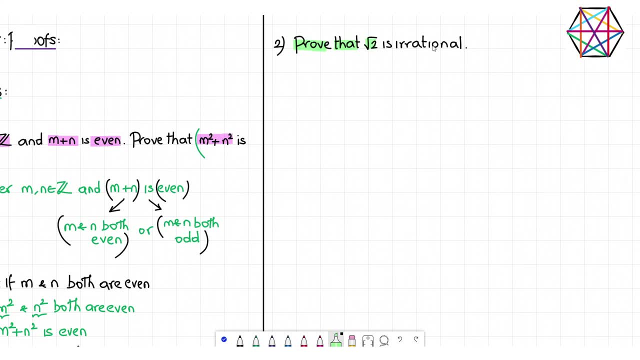 We have to prove that Square root of 2. Is irrational. We have to prove that square root of 2 is irrational. It's a problem of historic significance. Okay, it's a very, very important problem. The proof goes like this: 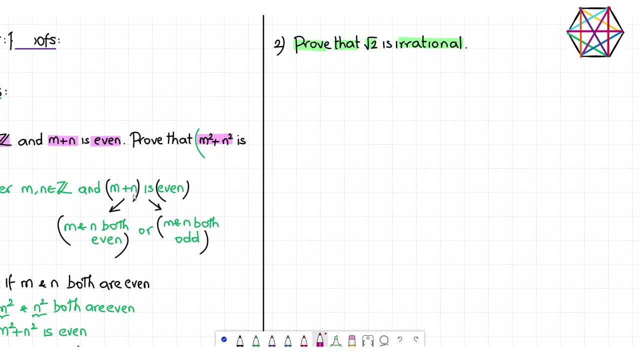 We are going to prove it by contradiction. You see, the previous problem is more like a direct proof. In a way, you can also argue it's a proof by exhaustion, because we are considering cases. You understand the meaning of proof by exhaustion. 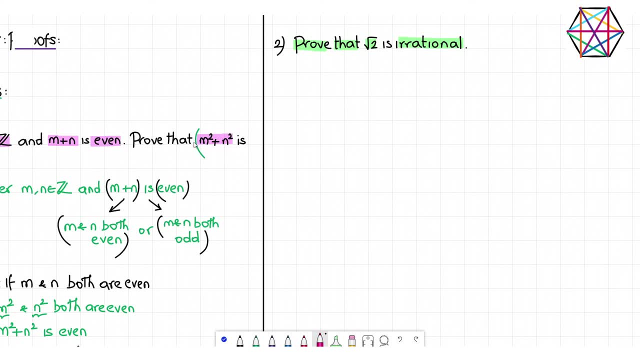 Exhaustion, Yeah, something like that. You break it down into smaller pieces- You know you will have to consider a few cases and you prove case by case. Whatever is the given problem, you break it down into four or five different cases and you solve or you prove case by case. 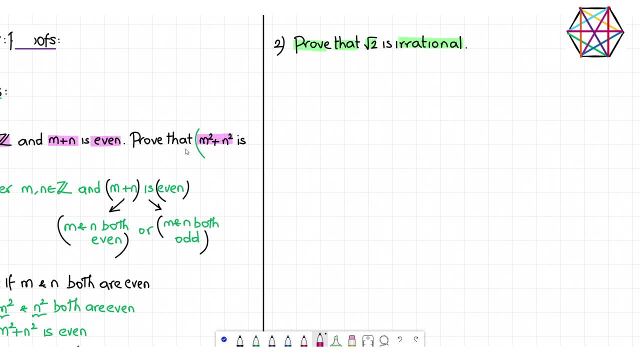 Did you get this? Okay? that is the meaning of proof by exhaustion. Yeah, Yeah, Yeah. Direct proof is Yeah, Yeah. You see an example. you will know There are some problems which will have shades of both. First problem is a very good example. 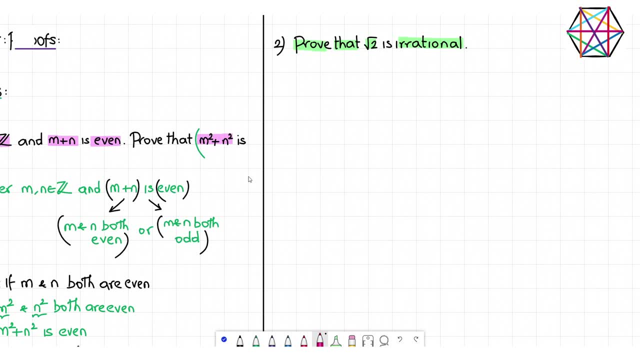 Okay, first problem: In a way you can argue: it's direct proof Also. you can, since there are some cases you can also argue: it is proof by exhaustion. Are you getting it Okay? so direct proof means something is given. 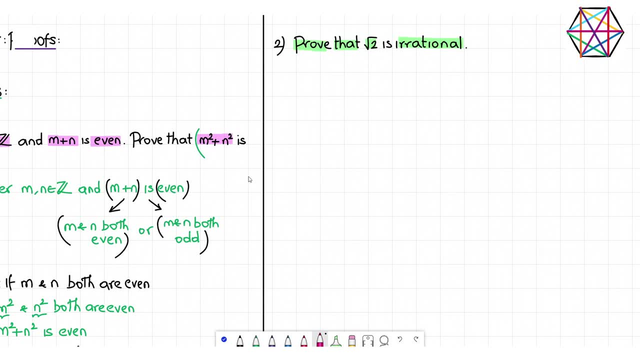 We are asked to prove. Okay, you're not taking any roundabout approach. Whatever is given, you start from there and you know, apply whatever is the relevant theorem or result. You can take a little bit of formula and do the math. you get the answer. 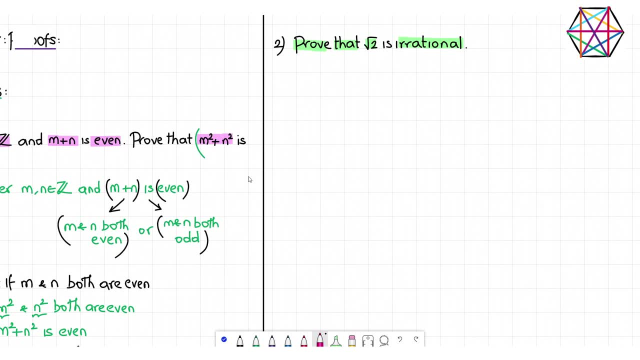 That is the meaning of direct proof. Right Right now, in second problem, we are going to see an example of indirect proof, particularly proof by contradiction. It's a classic proof. Take this: It's proved by. this is the best example of proof by contradiction. 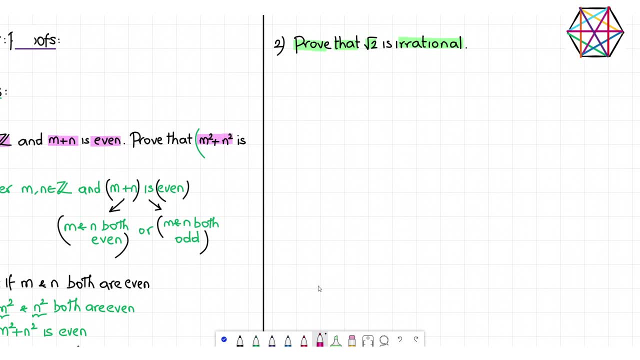 Okay, Okay, And it's also a very important problem. Listen. Prove that square root of two is irrational, Rational Fine. We are going to prove. prove it by contradiction. Let's assume the contrary. That is the first step in proof by contradiction. 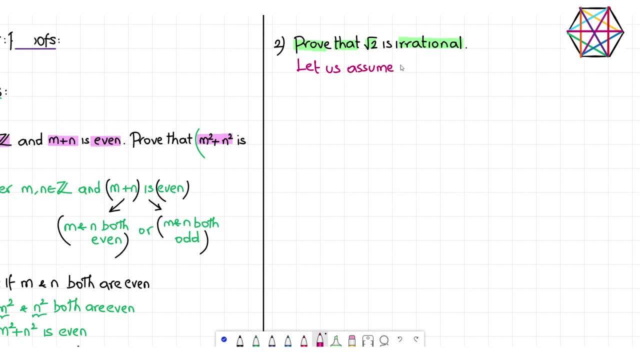 Let us assume The contrary. Let us assume, by contrary, Let us assume the contrary- that Square root of two is rational. let's assume the contrary, that square root of 2 is rational. if square root of 2 is rational, you know what is the meaning of it. what is the meaning of it, you will be able to. you know what. 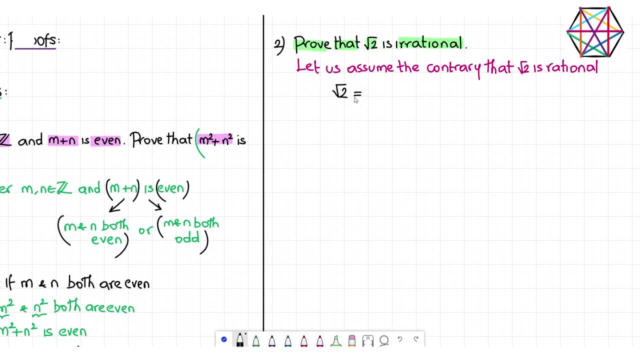 is a rational number. what is yeah in the form of yeah? so square root of 2 can be written in the form of p by q, where p and q both of them are. what is it? p and q? both of them are what integers, and q is non-zero. p and q, both of them are integers and q is non-zero. this is. 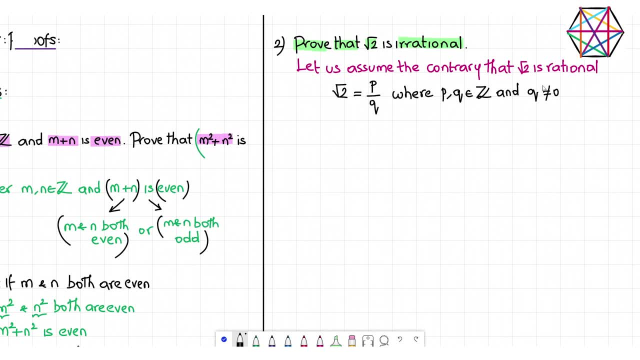 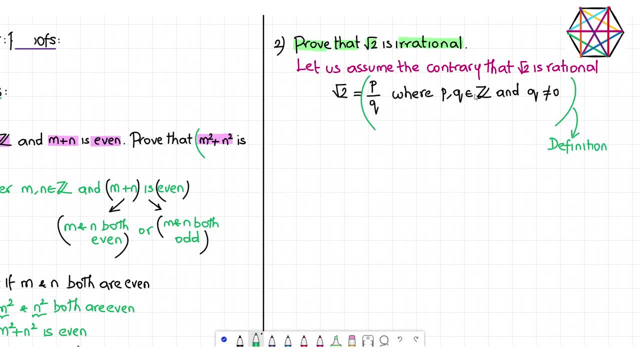 can be written in the form: p over q, where p and q- both of them are integers, where q is non-zero. this is called rational number. did you understand this? is that clear, yes or no? okay, so this is the definition of rational number and we are assuming that. 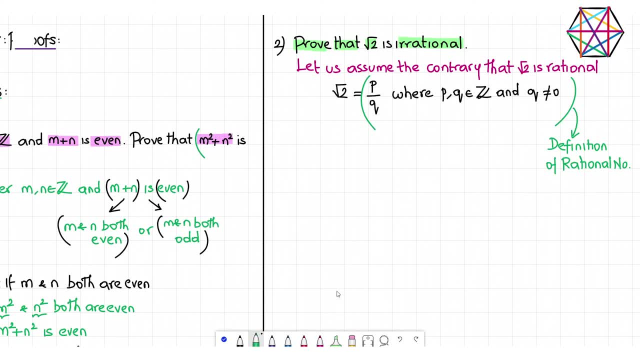 square root of 2 is rational. let's see what goes wrong if you assume that. okay, now, since square root of 2 is taken to be rational, which is p over q, i'm going to square both the sides. i'm squaring both the sides of this equation. what is square of square root of 2? 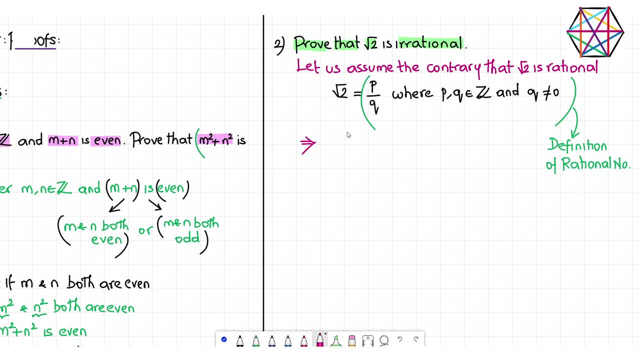 and one more thing, i'm assuming listen. one more thing. sorry, it's a very important point. i should have added: okay, where p and q are rational integers and q is non-zero, right? and also also let us assume that p and q are co-prime. what's the meaning of it? also let us assume that p and q are. 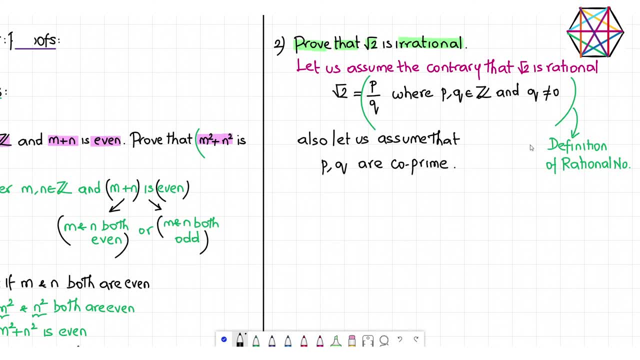 co-prime. what is the meaning of it? okay, by the way, this is the definition of rational number. this is not. this statement that i just now wrote is not definition. it's, it's not part of definition of rational number. definition of rational number is only this much. what you see within the green. 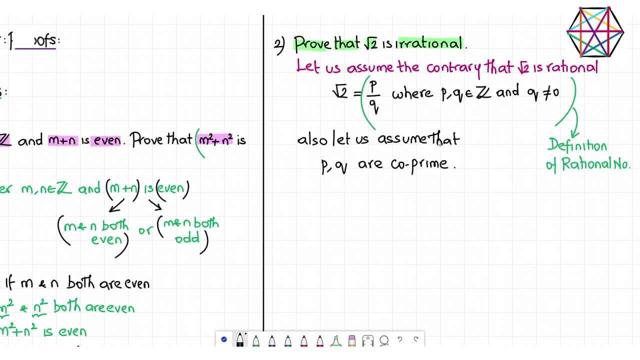 bracket. what i wrote here is like an additional condition. we are assuming, but you don't have to worry. like you know, are we not simply assuming things? okay, out of nowhere? you don't have to worry like that, because it is always true. you know what is the meaning of co-prime. 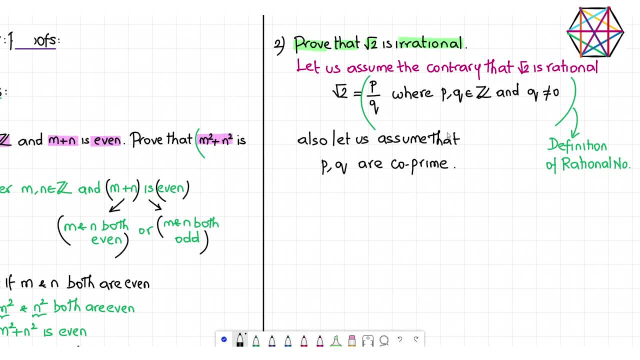 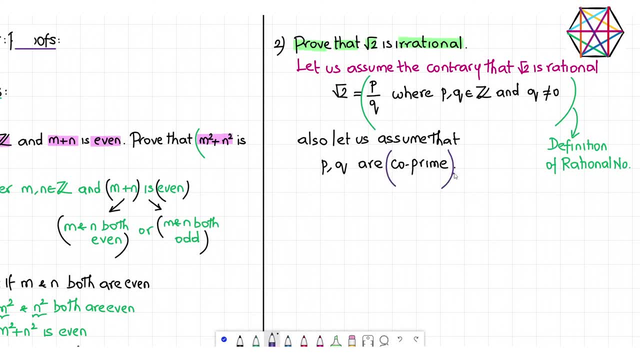 co-prime means no common divisor or factor, whatever you want to call it. no common divisor or factor, whatever you want to call it. no common divisor, except of course one is always there. no, except one. did you get this? no common divisor, except one example: 18 and 25 are co-prime. yes, i know, is 18 a prime number? no, is 25 a prime? 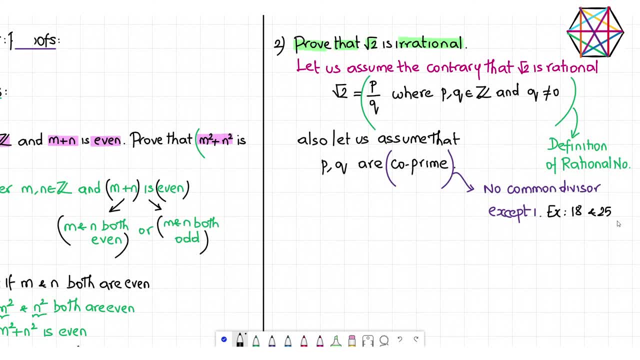 number. no, neither of them is a prime number, but still we say 18 and 25 are co-prime because they have no common divisor except for one. one will divide everything. okay, we can't help it. okay, except for one, there is no common divisor. did you understand this? okay, great, so now you understood. 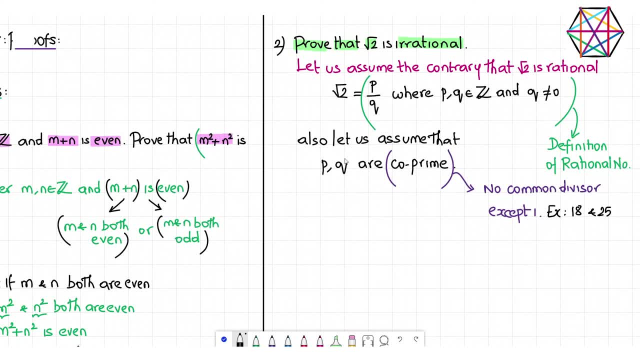 the meaning of co-prime. so why are we allowed to assume this? why are we allowed to assume that p and q are co-prime? you see, very simple. yeah, two numbers- wait, two numbers cannot be prime factor of each other unless those two numbers are one and the same. it is impossible. 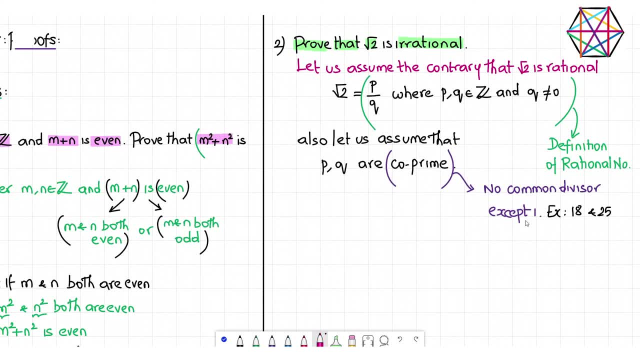 you are basically saying p and q are prime factors of each other. two numbers can never be. two distinct numbers can never be prime factor of each other. do you get this? five is a prime factor of 10. 10 is not a prime factor of five. first of all, 10 is neither prime nor it is a factor of five. do you get this? so, unless those, 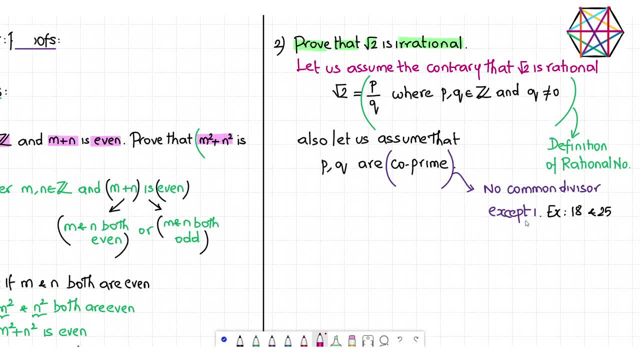 two numbers are equal. two numbers cannot be prime factors of each other. did you get this okay? so now answer my question. why are we allowed to assume that p and q are co-prime? how can you simply assume things like that? how can you simply assume things like that? 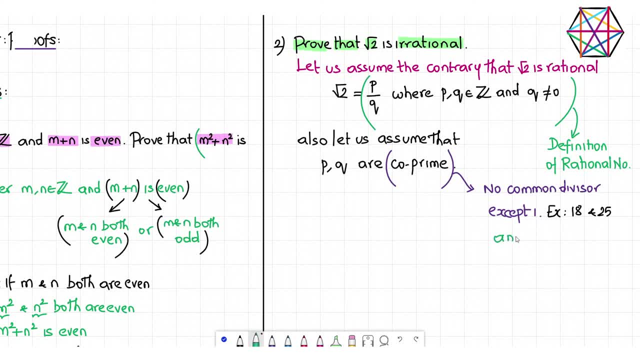 you see, i told you that square root of two is rational number. that is something we are assuming. rational number means both p and q are integers. q is non-zero, all that is fine. i am also assuming something extra: that p and q are co-prime. how is that assumption justified? 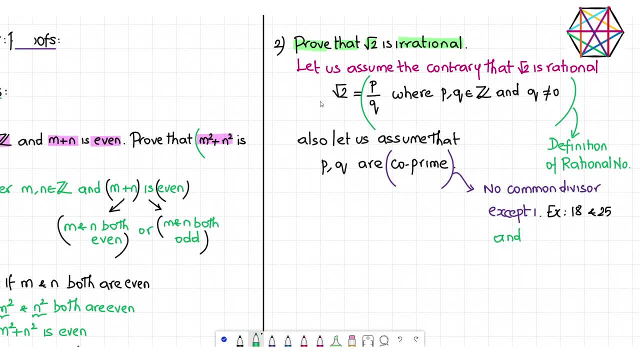 i'll explain how. forget about this problem. just forget about this problem. i'll just explain something in general. is this a rational number? forget this example, forget this problem. look at the definition of rational number and based on that, you tell me: is this a rational number? yes, it is. numerator p is a rational number and the numerator p is a rational number. 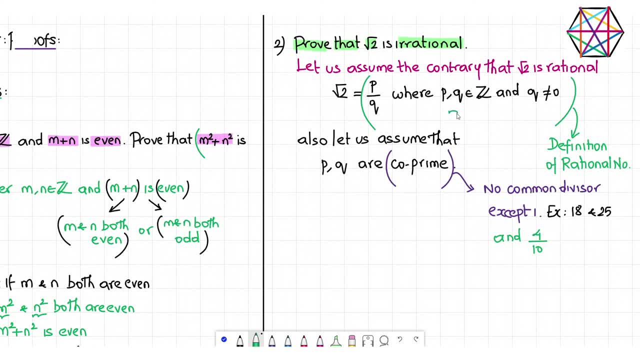 and the denominator q is an integer. both of them are integers and denominator is non-zero. yeah, it's perfectly satisfying that, given statement, it's a rational number, no doubt. okay, so 4 by 10 is a rational number, no doubt, but can you say that here, in this example? can you say that p and q are? 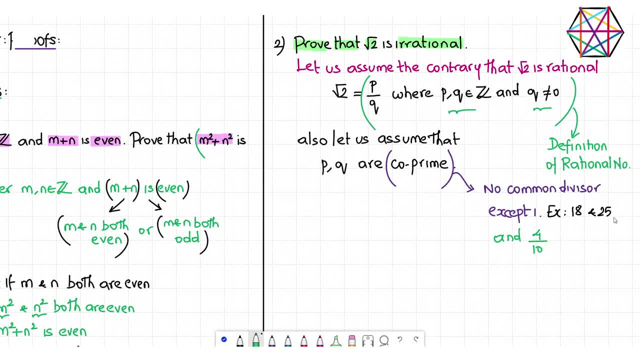 co-prime. can you say that p and q are co-prime? definitely not, definitely not, because two divides both numerator and denominator. i said the you understand. i said there is no common. yeah, yeah, i said there is no common divisor except for one. right, i told you that there is no common divisor except for one. 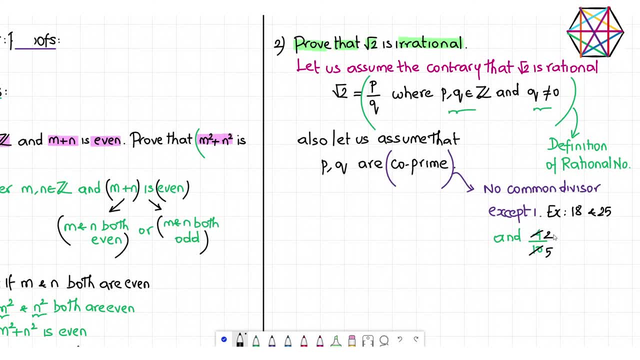 whereas what we have here? we have two, two divides, both numerator and denominator, and after cancellation, what do we get? we get two over five. now, what is this? you can certainly say now, p and q are co-prime. now you can certainly say anything will divide two and five simultaneously. nothing will, except for one, forget about one, okay. 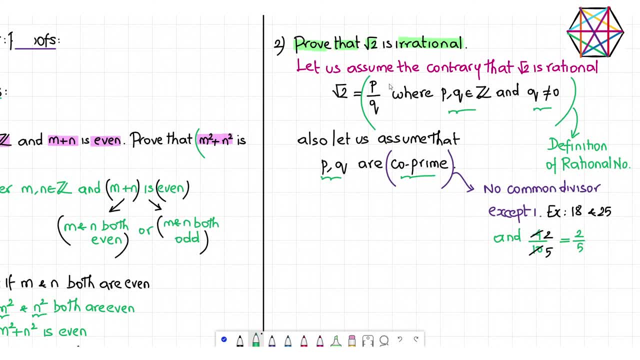 did you get this? so even if this rational number p by q is not co-prime, we can perform this cancellation and make sure that they are co-prime. does it make sense now? yes, exactly, okay. so what i'm trying to say is: i'm simply assuming that p and q are co-prime, right? 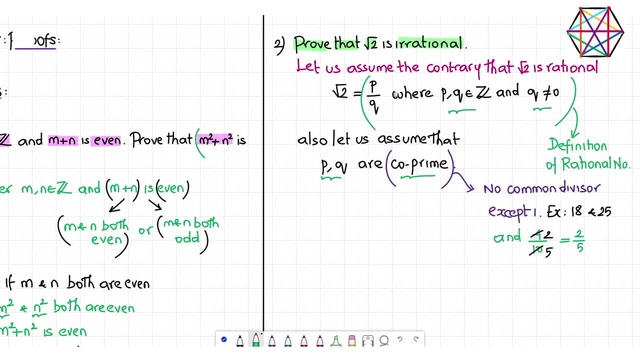 my assumption is justified because, even if they are originally not co-prime and we can perform this cancellation and we get the same fraction with the same value, but it looks like it's not different. instead of looking like four by ten, it'll look like two by five. now that, two by five. 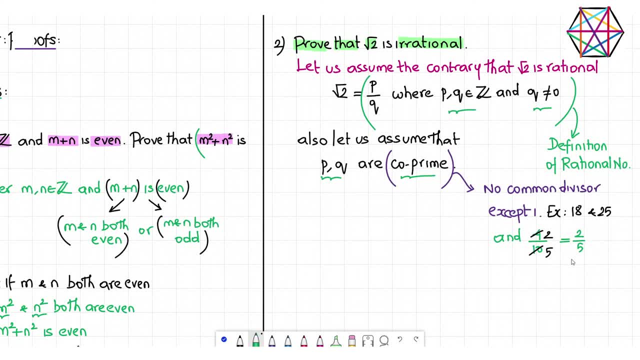 is my new p by q. that is not, that is not. no, it doesn't matter. you see, it doesn't matter. after we simplify the simplest form, whatever fraction we obtain, that numerator, i call it p and that denominator, i call it q. it's just a name we are giving for numerator and denominator, you call it. 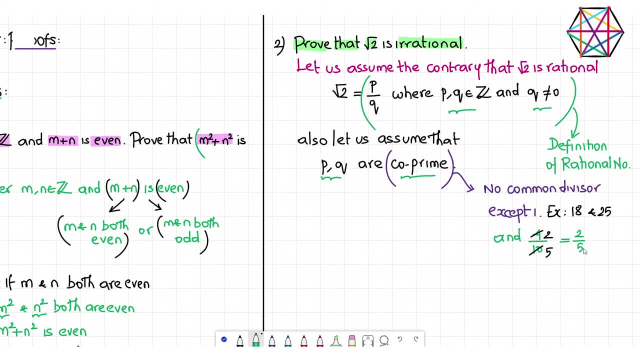 a, b, c, d, anything. it doesn't. no, we don't even know what that value is. we are simply assuming something. you see what? whatever value p over q is, whatever value p and q are, we perform the cancellation after we. your only concern is after you perform the cancellation. you should be, you shouldn't be. 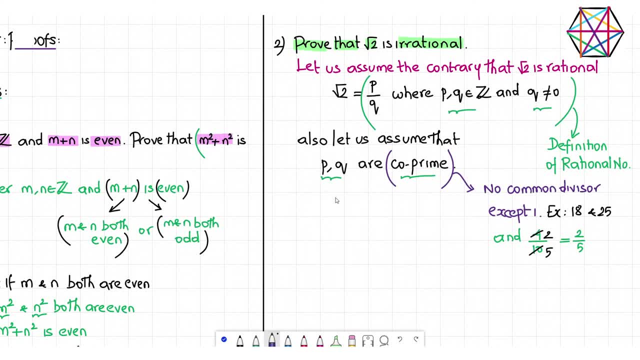 writing it p and q anymore. you should be writing it, say: uh, a by b. is that your concern? is that your point? is that your point? okay, now, this is where i want you to understand something: that these p, q, a, b, these are dummy variables. don't take them too seriously. these are placeholders. 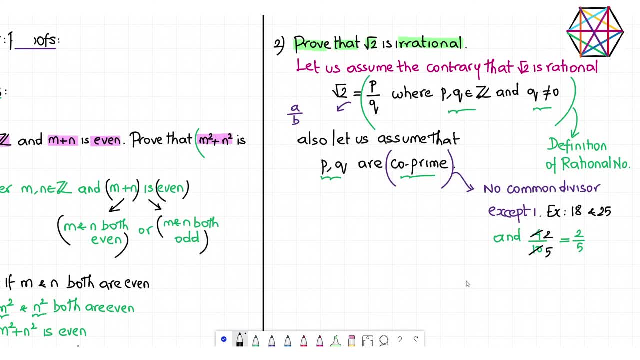 you understand these are in primary school. you must have solved problems like this. okay, fill in this empty space for me with a suitable number. you know it is two. right, you know what purpose that triangle is serving? it's just a placeholder. it's a dummy thing. it doesn't mean anything. no, no, no, no, no, wait, wait. 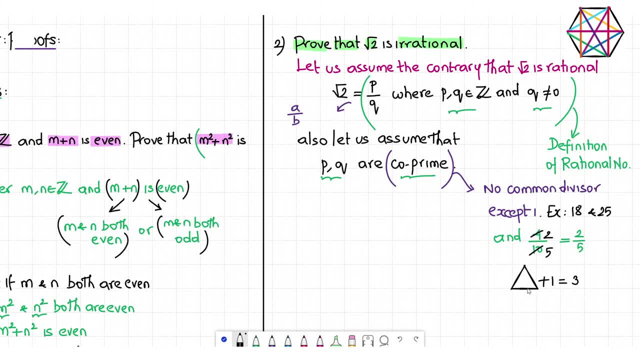 wait, it's just a dummy thing. wait, i'm not done this. triangle is just a dummy thing. okay, now would you call this a different problem? is this a different problem compared to the previous equation? no, instead of, instead of triangle, we have a different problem. so we have a different problem. so we have a different problem. 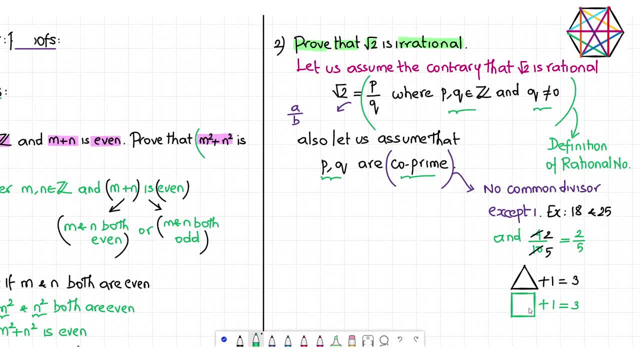 square. is that a problem? no, it's not an issue at all. it's just a dummy thing. it's a placeholder. so likewise, you're telling me that, okay, p and q, they may have something in common. you have to cancel them, and after that we get the same fraction, which looks different. we should call it a by b. 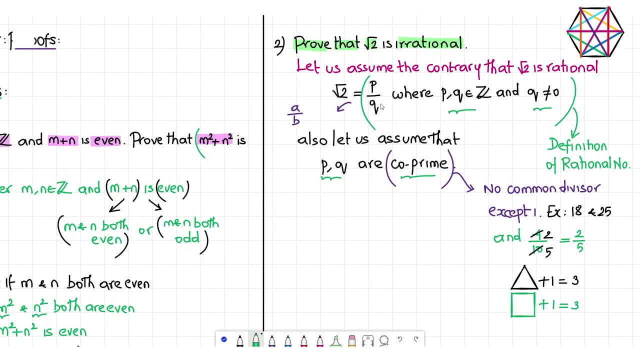 we don't have to complicate things. even that new fraction, we can simply call it p by q, i'm already assuming that they are co-prime. i'm already assuming that, and, and my justification is, i'm not wrong in assuming that, because even if it is not true, i can always make it true, and after i make that thing true, then 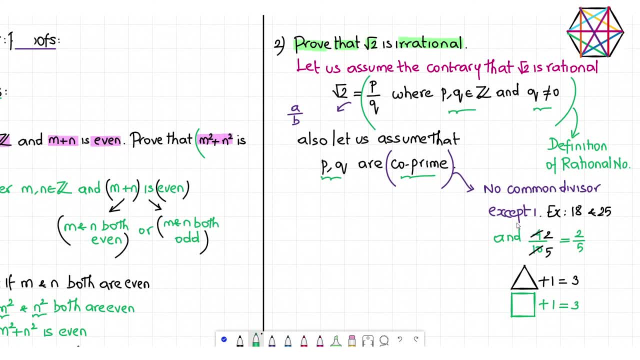 that fraction. i call it p over q. yeah, i don't know, you didn't get it. you didn't get it exactly. there you go, They are, they are, they are the same fraction. yeah, Not in the form of fraction. Oh then, then we can't do it. 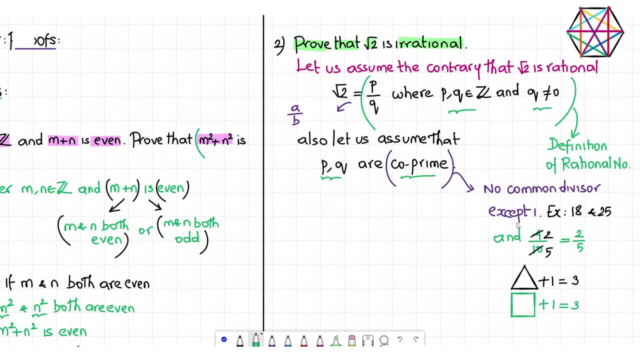 Then your point is valid. Yeah, then it is valid. I'm talking specifically about this fraction P over Q. Do you get this? Exactly exactly the point. Exactly the point. Listen, first of all, I'm not even going to carry out this act of canceling and simplifying. 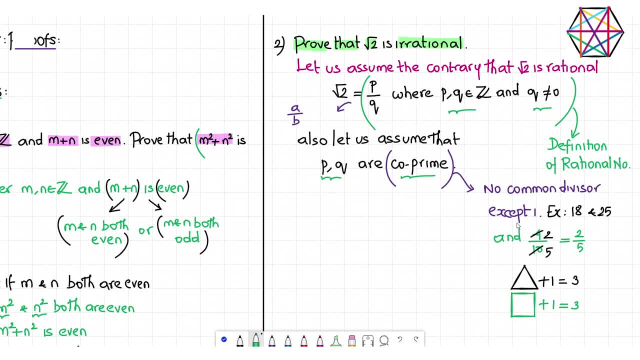 and all, Even to begin with, I will simply assume that it's in. you know, it's in simplest form. I will simply assume it's co-prime And I have already proved that. why you cannot question how. how can I simply assume things? 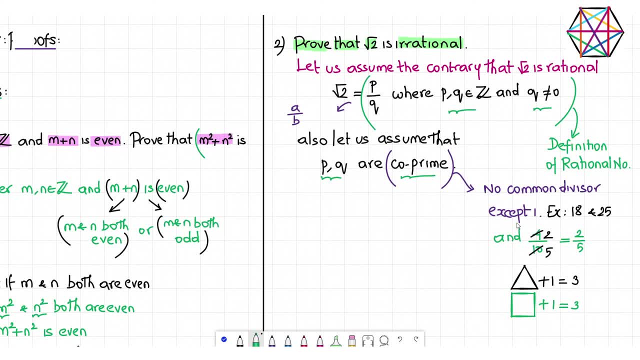 Because I told you that I can always make it happen. I can always make it true. Okay, so that part I'm skipping. Okay, I'm already assuming that P and Q are co-prime. okay, that's it, yeah. 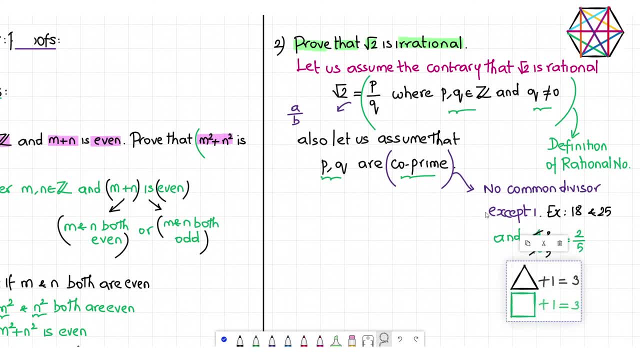 So now, okay, now, till here, it's all fine. okay, Now how to prove it, This equation, we are going to square both the sides. What is square of root 2?? What do you get when you square square root of 2?? 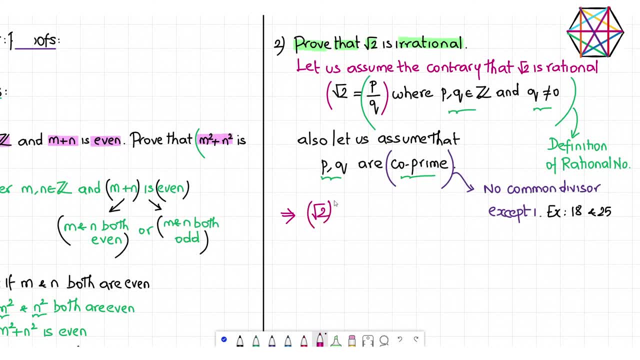 Okay, What do you get? And what is that? You don't even have to do that, It's a roundabout. What is that? You see, squaring and square root are opposites of each other. right, They both are opposites of each other. 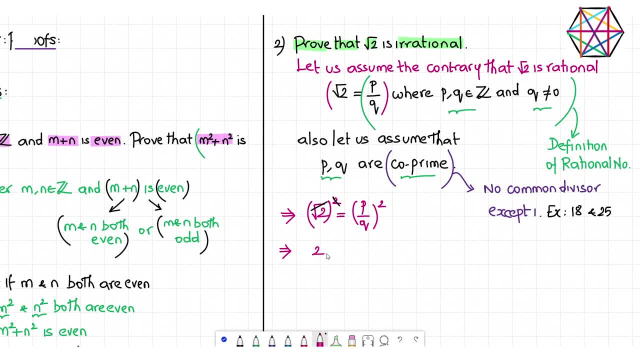 We will get 2, we will get 2 equals P squared divided by Q squared. Did you get this? Yeah, you got this. Now, what is? yeah? how is it related to the problem? You will know once I am done with the problem. 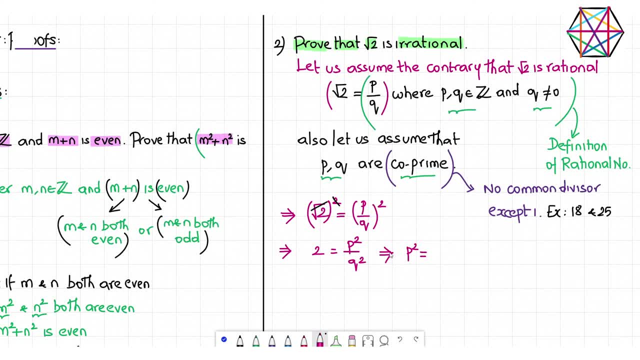 Towards the end, you will know. Okay, Okay, okay, yeah. so p square equals 2q square. that's a very valid question. okay, this assumption makes sense because i called it proof by contradiction. so assuming that square root of 2 is rational it. 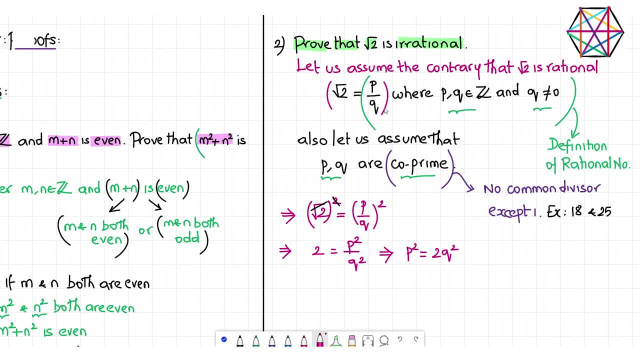 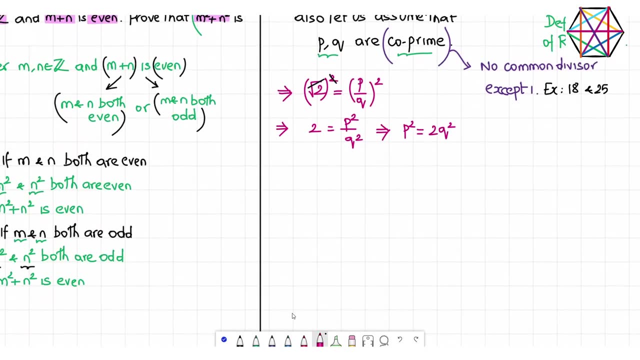 makes perfect sense, but why am i assuming it to be a special type of rational, not just a rational? why are we assuming something extra? you will understand okay. so p square equals 2 times q square after you cross multiply. yes, p square equals 2 times q square. yeah, now tell me what. 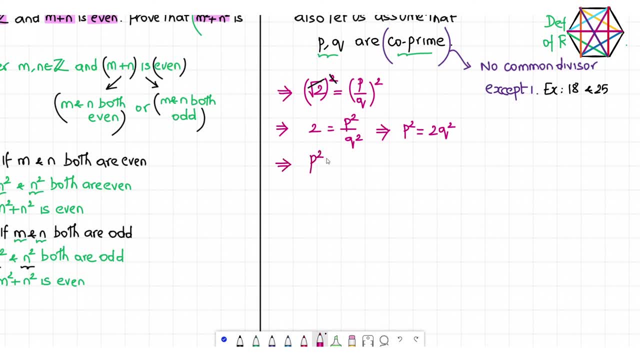 kind of number is p square? what kind of number is p square? you tell me, look at this, it is 2 times something. i don't know what that thing is. that doesn't matter the moment. you see, 2 times. what kind of number is p square? 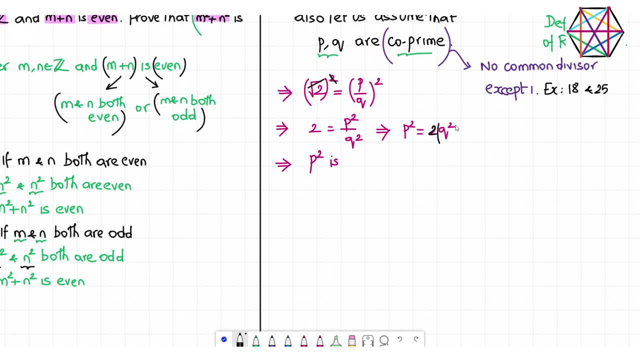 yeah, 2 times of q square. let that q square be even or whatever it is. the moment you multiply by 2, by definition even number is multiple of 2, right? so what is 2 times of q square? it's a multiple of 2.. so what is p square? it's a multiple. 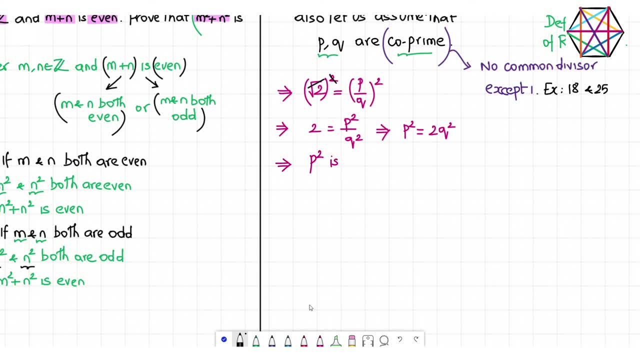 of 2. so what is p square even agreed, okay, p square is even, p square is even and p square right. if p square is even, what can you say about p? you only tell me, if p square is even, what can you say about p? we know that p is an integer. we know that p is an integer. yeah, yes. 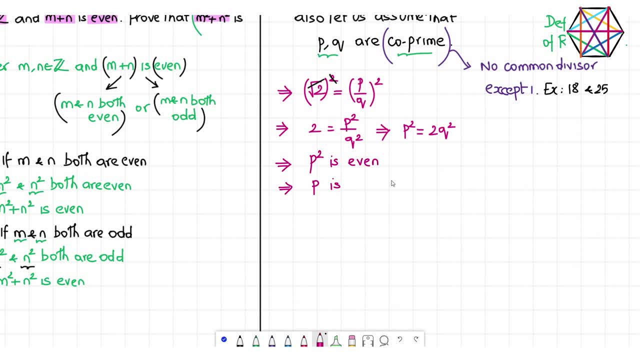 it has to be even. you see, you have only two possibilities. we know p is integer. either p is even or it is odd. if p is odd, odd multiplied by odd will be odd, always, always. three times, uh, three ten, i mean eleven times eleven. are you getting it? odd multiplied by? 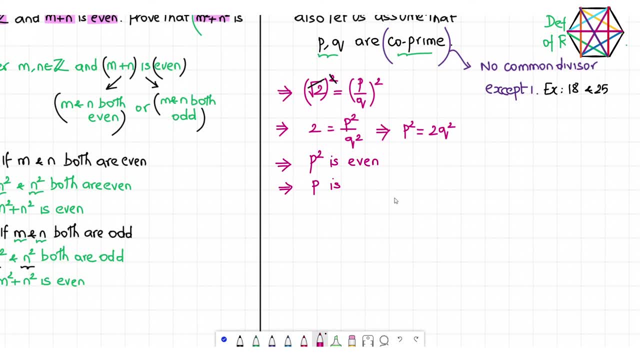 odd will always be odd. even multiplied by even will always be even. so the only way, exactly. okay, but that's not exactly, you know, relevant here, but it's a valid point. so, since p square is even, what can you say about p even number? now, if p is even number, don't you see that p can be written as: 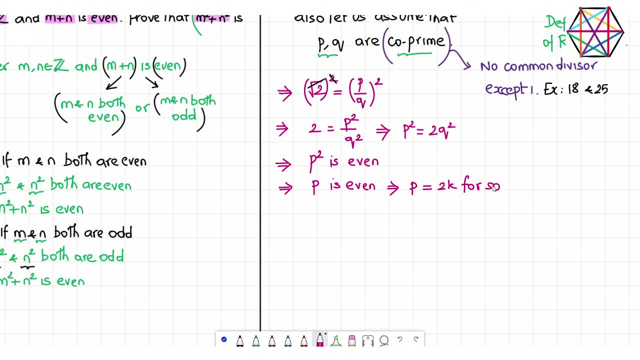 2 times k for some integer k. what is the meaning of even number? it's a multiple of 2. which multiple of 2? i don't know. it may be 17th multiple of 2 or 28th multiple of 2, i have no idea. it is some number k, some integer k times 2. 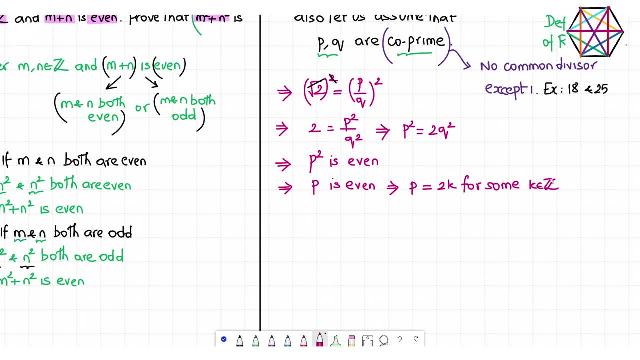 make sense. you didn't understand this equation. yeah, p is even, even means it is a multiple of 2.. right now, which multiple of 2? we don't know. it can be 17 times 2, it can be 20 times 2, it can be. 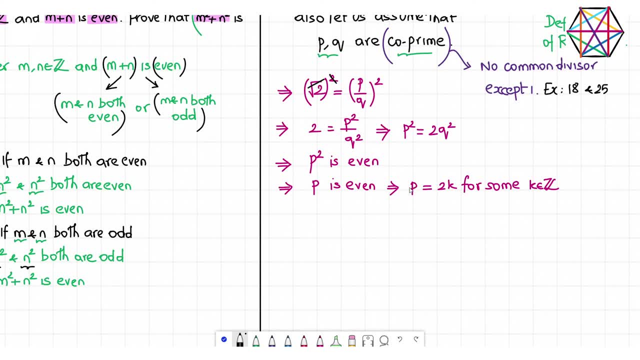 33 times 2. we don't know which multiple of 2 it is. i know that p is even. therefore, it is some integer times 2.. i have no idea what that integer is. it is some integer times 2, yes or no? yes or no? 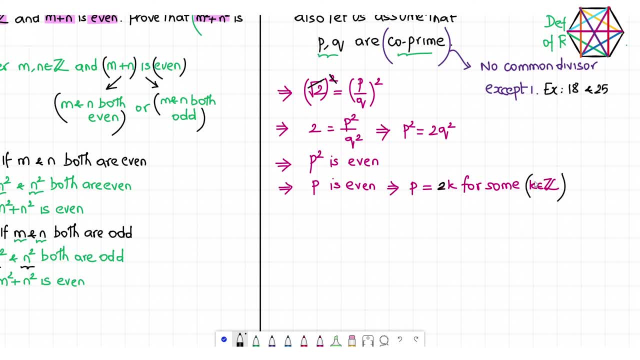 no, if it's fraction times 2, it need not be an even number. okay, you see, think about it. okay, what is 2 times of 1.5? it's not even number. forget about this. it can be even worse. what is 2 times of 1.4? 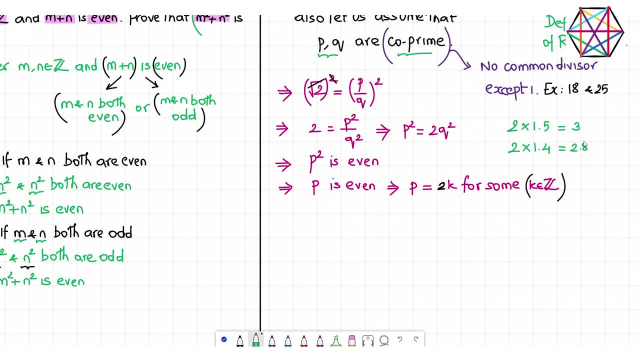 2.8. it's not even the question of even or anymore. it's not even an integer in the first place. okay, so it is 2k, right, that k must be an integer. know, the option k must be an integer, right? okay, so now i'm going to use this. i'm going to use this in this equation. i call it equation. 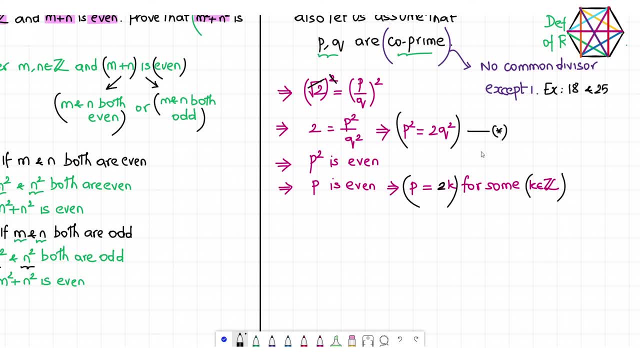 star. i call it equation star, i call it equation one. call it equation one, substitute equation one and equation star. substitute equation 1 and equation star. you know what we get? what do we get? p is equal to 2k, right, i'm substituting here, so 2k, the whole square equals. 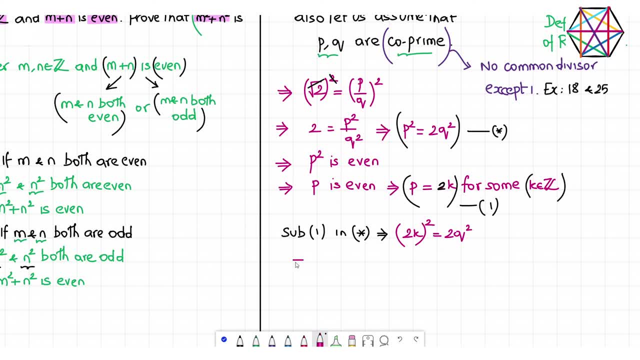 2, q square, right. so what is it? what is 2k? the whole square? is what? 4? and what is k square? k square, only just write it like: k square equals 2 times q square. did you get this? do we have any common factor in both lhs and rhs? we do. what is it 2? we can. 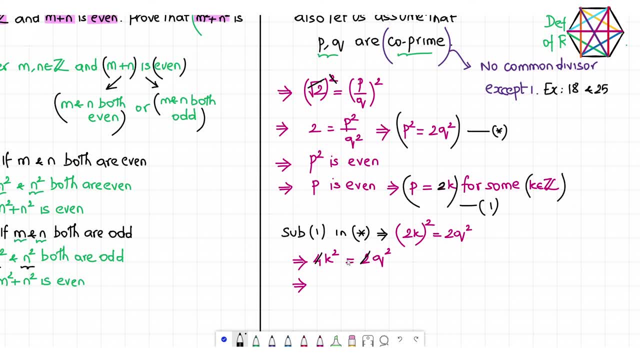 divide by 2. here that 2 will be gone. here that 4 will become 2, yes or no? so what do we get ultimately, we get q square equals q square equals 2 k square. q square equals 2 k square. did you get this? now, what is the meaning of saying q square equals 2 k square? what is the meaning of it? it? 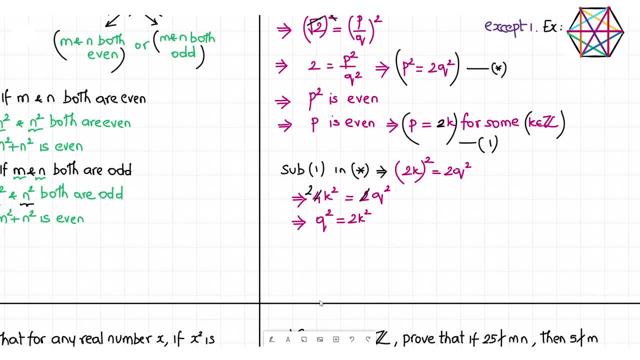 means what q square is. no, no, no, no, no, no, no. q square equals 2 k square. it means q square is even. it means q square is even because it is 2 times some k square. it's 2 times some integer, so it's even. 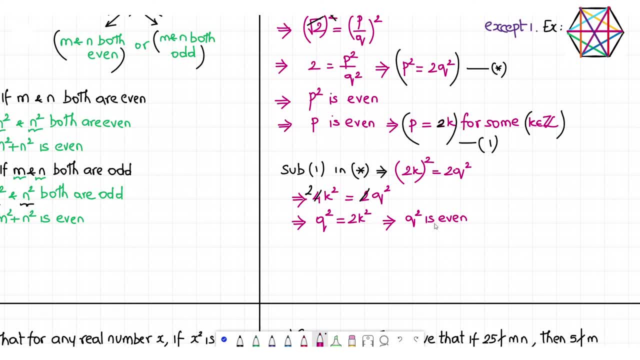 are you getting it? so q square is even. is that clear? yeah, so q square is even. if q square is even. i'm asking you the same set of questions once again, don't you see? i'm asking you the same set of questions. okay, if q square is even, what can you say about q? 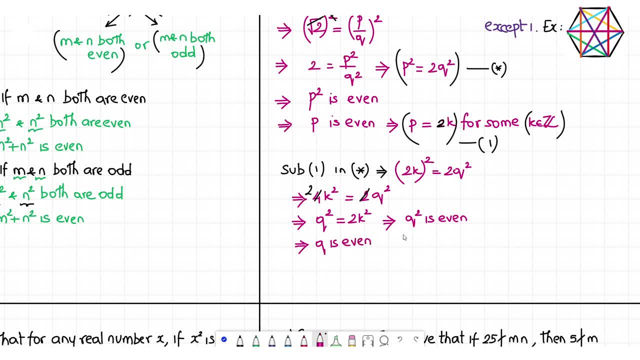 round. this is going to come from casing q is even, q is even right now. focus on this and this: if p is even, then p is a multiple of 2, obviously right, if q is even, then. So this implies 2 divides. it implies 2 divides both p and q simultaneously agreed, which 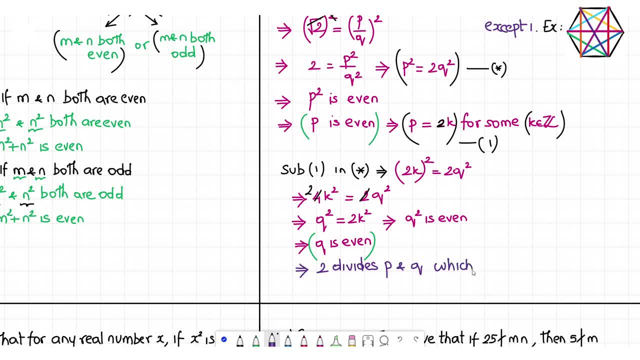 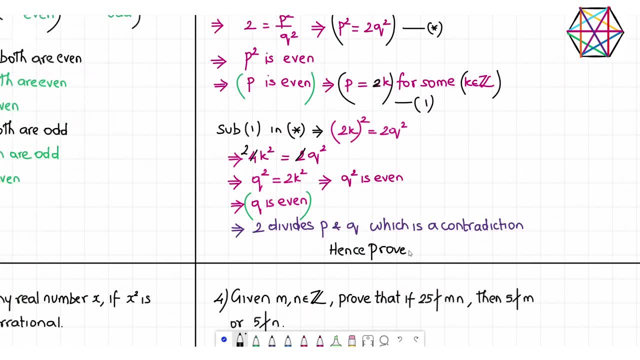 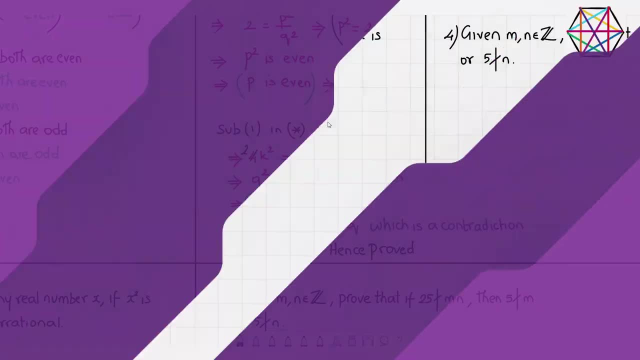 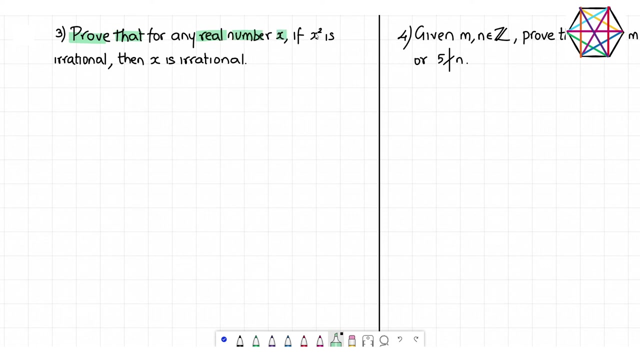 is a contradiction. You understand why it is a contradiction: Contradiction to our assumption that p and q are co-prime. Hence Prud'art claimed that square root of 2 is irrational. did you get this Sum number 3, prove that for any real number: x, x square. if x square is irrational, then 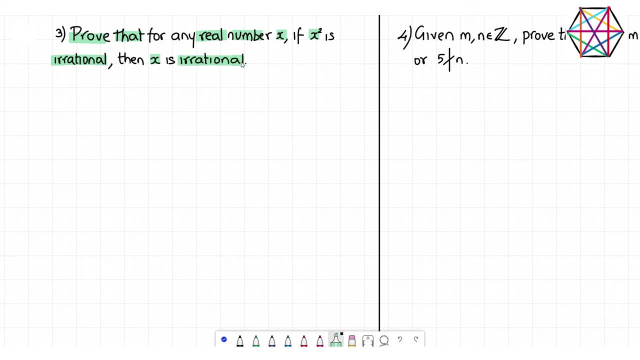 x is irrational. I repeat: prove that for any real number, x. if x square is irrational, then x is irrational. okay, Now here we are going to prove it using contrapositive. prove by contrapositive. Okay, I am writing it here we are using using proved by contrapositive. 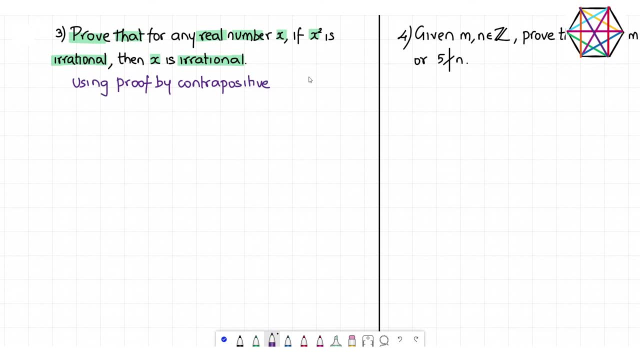 You know what is the meaning of proved by contrapositive? Okay, You see, we have this statement: conditional statement. you know what is the meaning of conditional statement, yes or no? what is it? take this: the nature of conditional statement will be like this: if p, if statement p is true, then statement q is true. this is 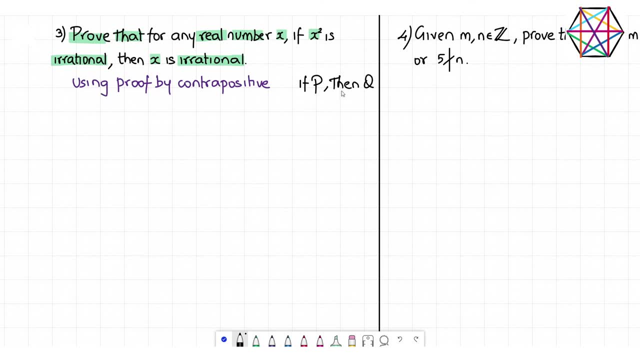 the nature of conditional, the whole thing is called as conditional statement. if statement p is true, then statement q is true right Now. when we are asked to prove this, instead of proving this, we can sometimes prove another statement which is equivalent to this. that is, another statement which is equivalent to. 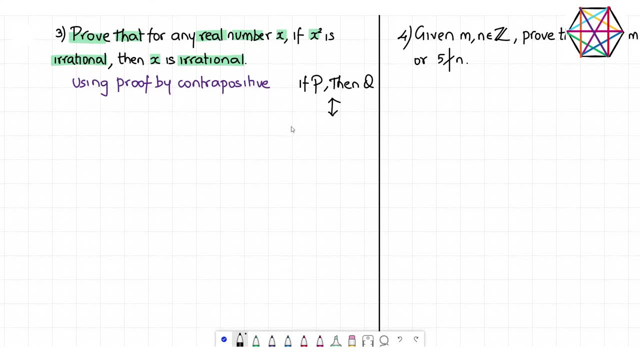 this, that is, if not q- I will explain what it is- then not p. I repeat: if not q, then not p. If not q, then not p. I claim that these two statements are equivalent. I claim that these two statements are equivalent, yes or no. 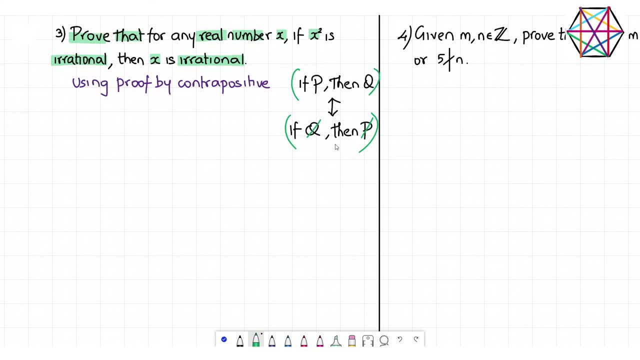 Did you understand this properly, right? So these two statements are equivalent. okay, So the second statement is called as second statement is called as the contrapositive of the first statement, or you can say they both are contrapositive of each other. 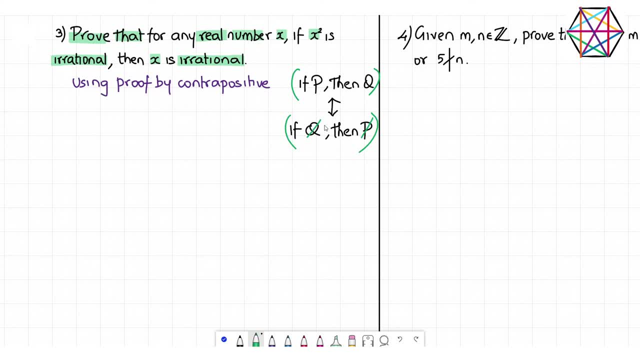 Is that clear? they both are contrapositive of each other. yeah, yeah, We don't have anything called as contra negative. no, okay, We don't have anything called. as you see, contrapositive is a statement which is like: 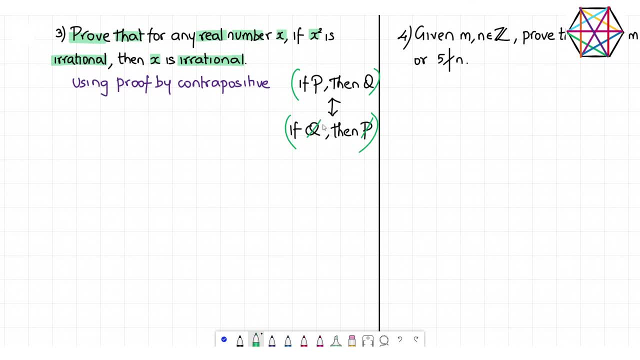 you know, saying the same thing in a different way, I am making a very silly comparison. I know it is silly, but it kind of helps. okay, In English it is like you know, you have active voice and passive voice, right, not? 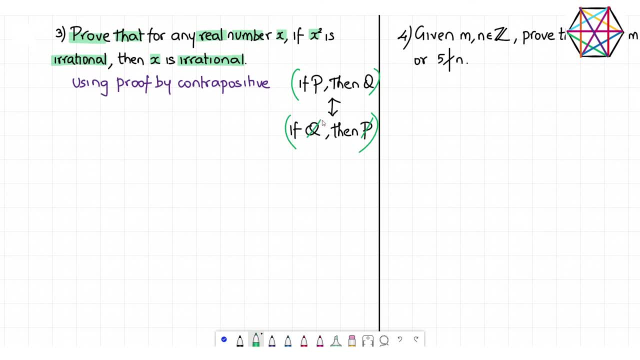 exactly. Just trying to draw a parallel. okay, something like that. you are conveying the same thing in a different manner. Are you getting it? okay? what to say? okay, I will just, I will give you a non-mathematical. 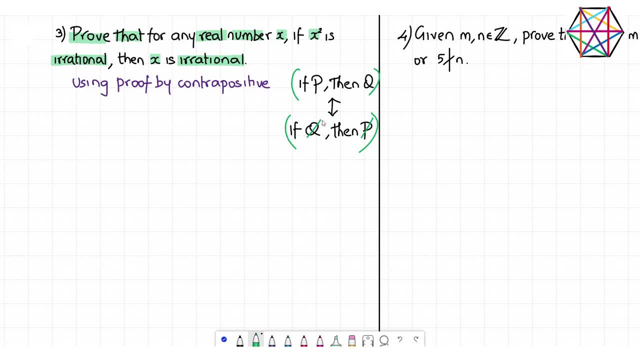 example: right, If this month is December? if this month is December, then this month has 31 days. okay, Listen, I am writing this statement, the original statement. I am writing: okay, If this month is December. no, it is okay, I purposely chose this. there is some reason. 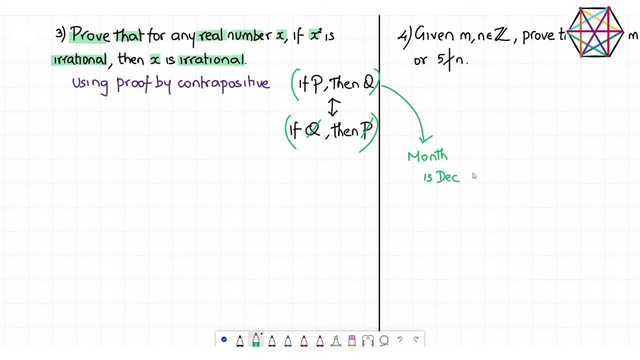 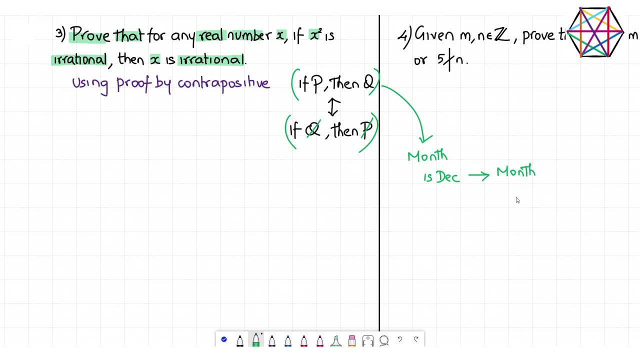 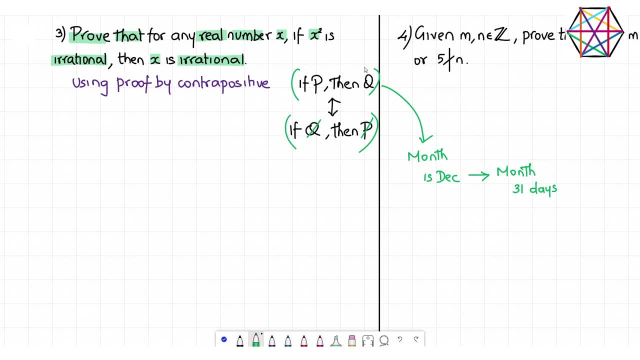 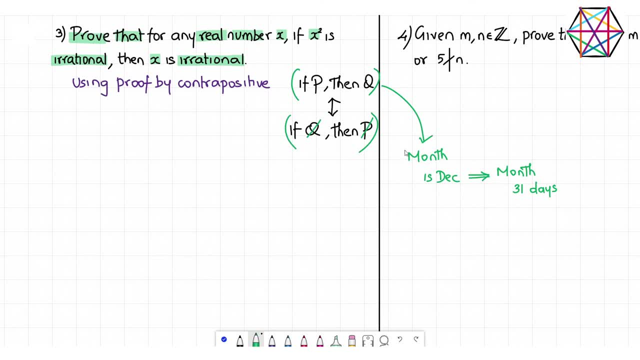 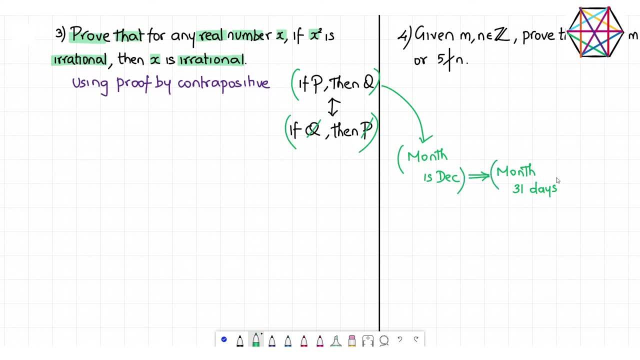 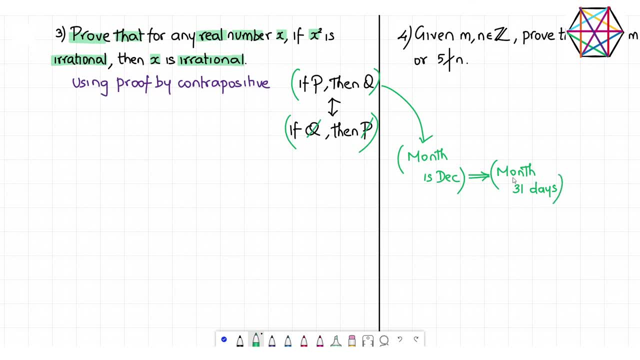 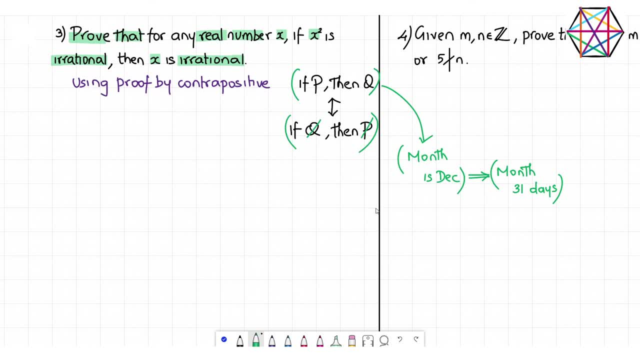 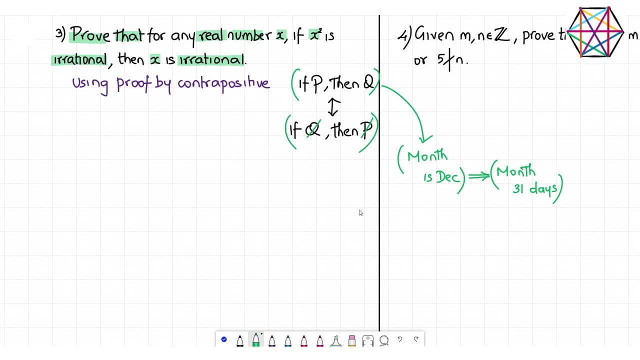 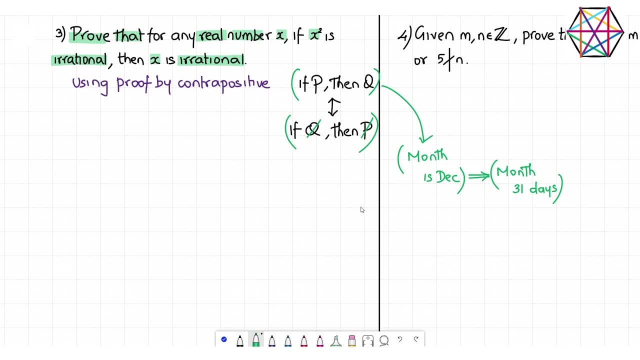 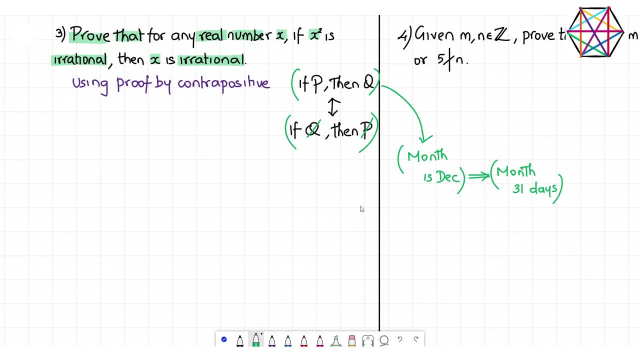 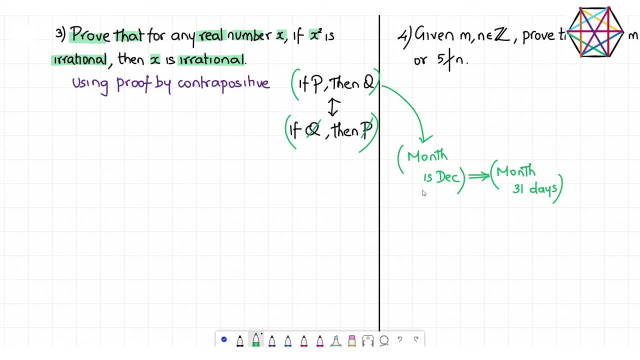 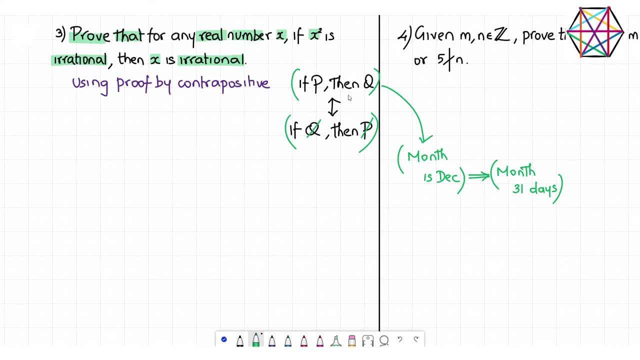 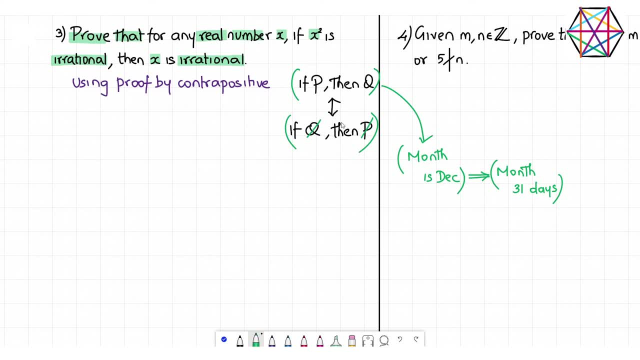 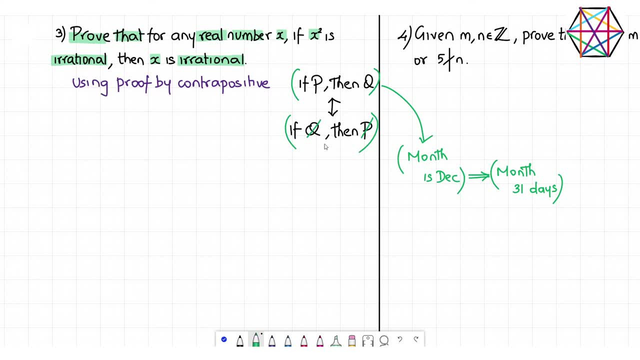 Okay. So if this month is December, then this month has 31 days. Okay. So if this month is December, then this month has 31 days. Okay, because it's equivalent, right? that is exactly what we're going to do here, so that's the meaning of. 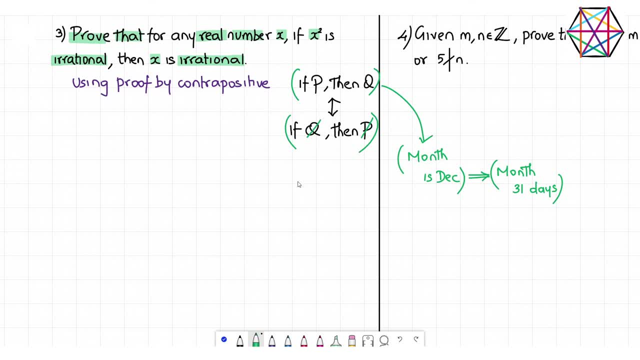 using proof by contrapositive. okay, check this first. write the contrapositive of the given statement first. let us write the contrapositive. this is the original statement, right? write the contrapositive of the given statement. what is the contrapositive? you know what is the given? 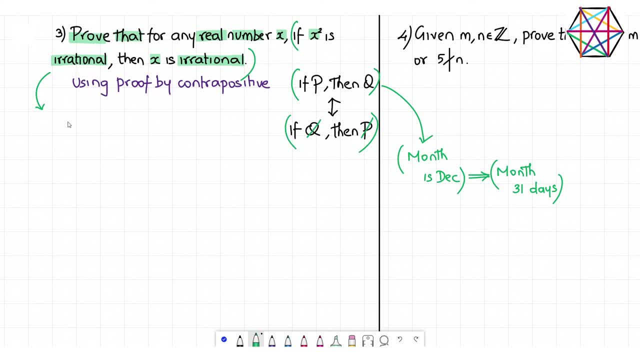 statement: if x square is irrational, then x is irrational. what will be the contrapositive? you tell me: come again. you know what you said. you know what you just said. you said: i'll write it down. you gave me this. you, my original statement is: if p, then q, and you gave me exactly this. if not p, then not q. this 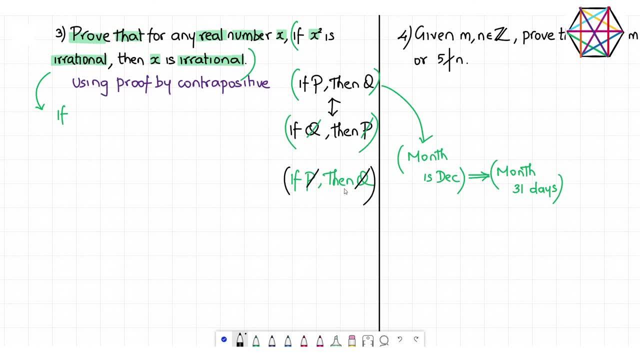 is exactly what you gave me. do you realize that? do you realize that? see what i have written here. this is contrapositive. this is not contrapositive. there is a different name for this. that thing we'll talk later. talk about it later. this is contrapositive. if not q, then not p. 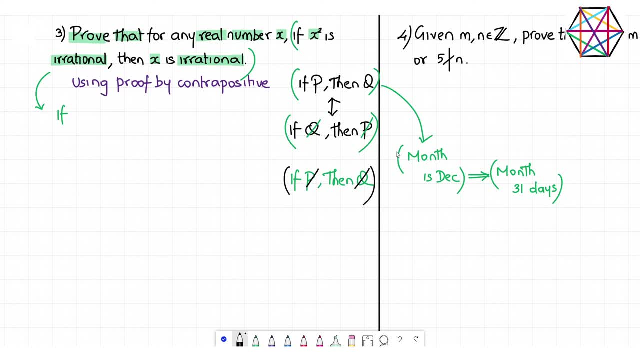 are you? you do you? do you understand this? listen? this is contrapositive. this is the original statement. this is contrapositive. what you gave me is: it is called as converse. i don't want to overburden you. it's called as converse. okay, you gave me: if not p, then not q, and you gave me: if not p, then not q. this is contrapositive. 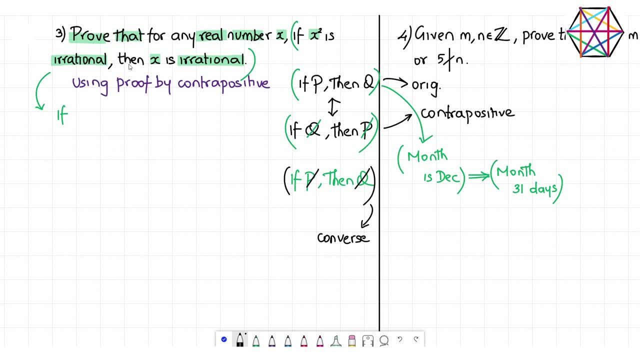 what is the statement? if x square is irrational, then x is irrational. that is the original statement. no, you know what you gave me? if x square is rational, you know what? what? what, what you just uttered? you uttered not p- then x is rational, that is not q. you apply your same logic over here, you. 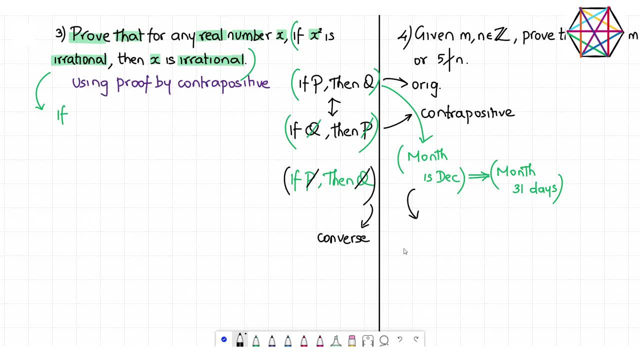 apply your same logic over here. if this month is not december, if this month is not december, then this month doesn't have 31 days. is that true? is that true? is that true? if this month is not december, then it doesn't have 31 days. is it true? no, it can be, jan it. 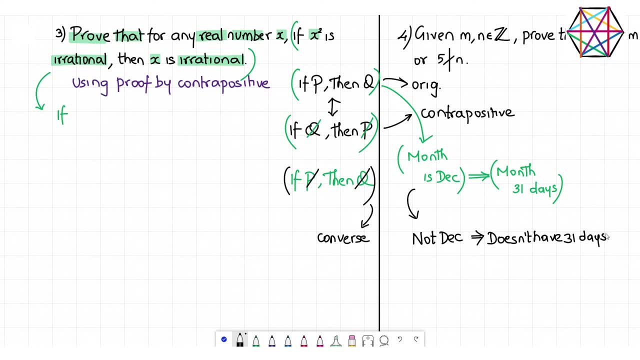 can be january, but it has 31 days, right, yeah, okay, so don't get confused between things. you got it. so what is the contrapositive of the original statement? what is the contrapositive of the original statement? what is the contrapositive of the original statement? 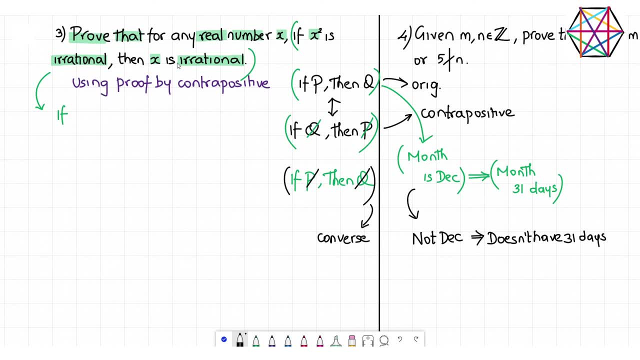 that is what you can either put: it's perfect, okay. you can put it this way: if x is rational, instead of saying: not irrational, simple rational, okay. so if x is rational, if x is rational, then what x square is is rational. if x is rational, then x square is rational. that's it. this is the. 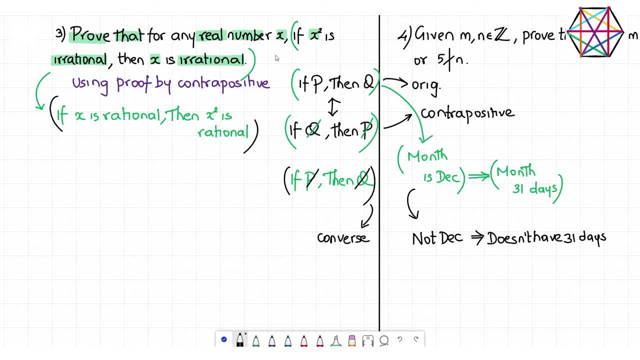 contrapositive of the original statement, the given statement. what you said was: if x square is rational, then x is rational. you, you gave me this right, okay. whereas i'm looking for this, this is the contrapositive. always remember: original statement. original statement and contrapositive are basically the same thing. they look different. 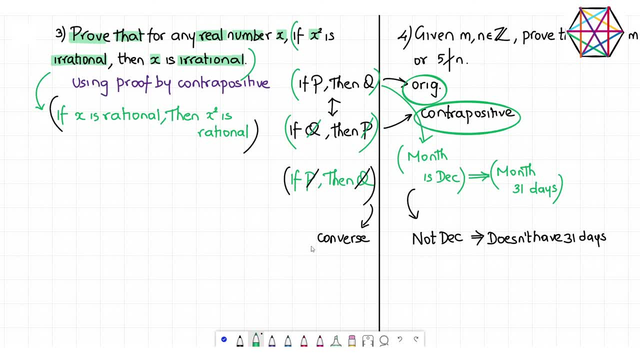 whereas converse is entirely a different thing. is that clear? yeah, okay. so instead of proving the original statement now, we are going to prove the contrapositive. okay, so i'm going from here to here. if x is rational, okay, if x is rational, what is the meaning of it? you know the definition of rational. 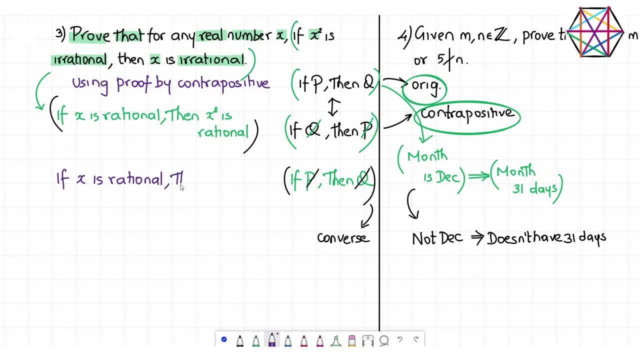 what is the meaning of it? if x is rational, then exactly x can be expressed in the form of p by q, where p and q both are integers and q is non zero. p and q, both are integers and q is non zero. okay, on 0 then, what is x square? it's p by q, the whole square, that's p by q times p by q. that will turn. 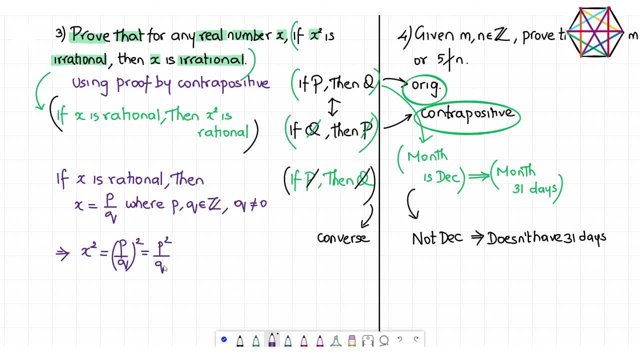 out to be what p square divided by q square. now, now think about it. what can you say about p square and q square? are they not integers? of course they are. if p and q themselves are integers, p square and q square, both of them are integers beyond doubt, and i have to also prove that denominator. 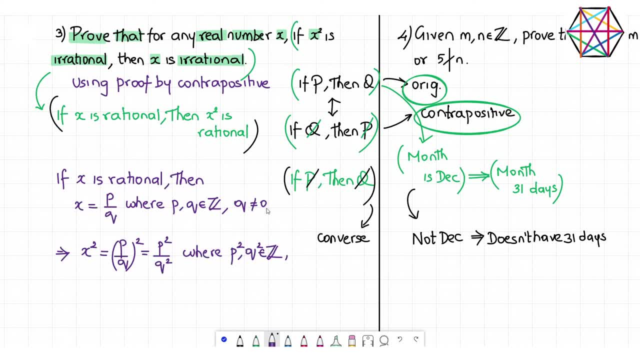 is non-zero. once again, it's pretty obvious: if q is non-zero, if a number is non-zero, even the square of the number is non-zero. so you know what did we prove? we proved that x square is rational. if x is rational, x square is rational. did you get this? hence proved. 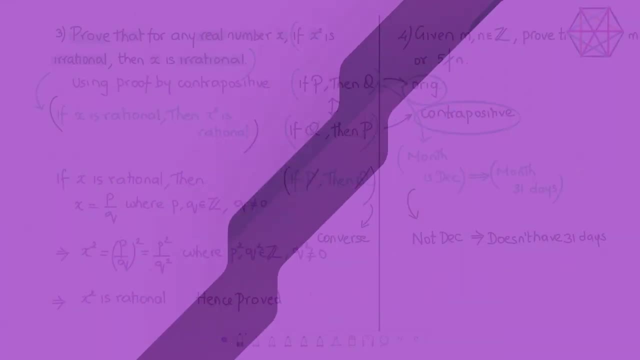 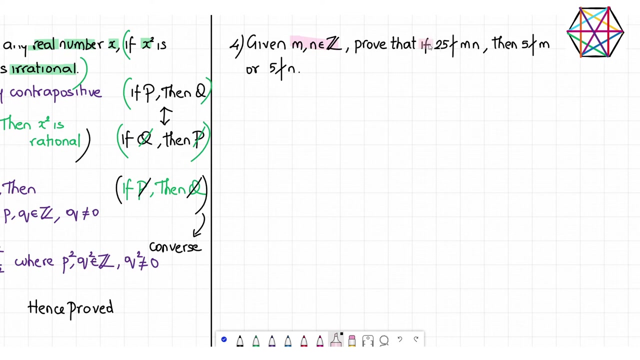 did you understand this problem? number four: given that m and n, both of them are integers, it's given. then prove that if you know what is the meaning of the symbol, the vertical line, and slash what is that you don't know. okay, does not divide. i'll explain. if 25 does not divide m, n, then 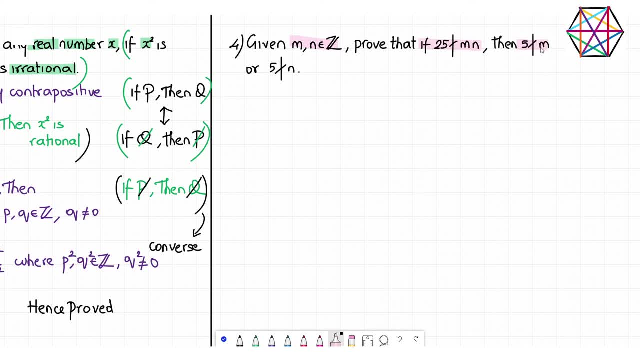 prove that five doesn't divide m or five does not divide n. okay, first thing, i'll explain. first thing. let me explain. this means, or i'll okay. this symbol means does not divide. this symbol means does not divide. did you get this? let me explain. this means: does not divide. 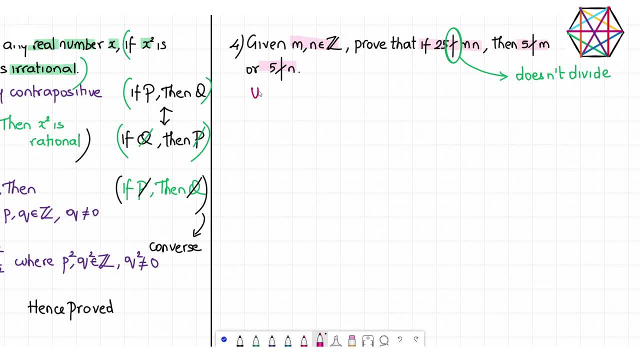 doesn't divide. okay, even here we are using proved by contrapositive. proved by contrapositive. did you understand the statement? m and n, both of them are what integers it's given. both m and n are integers and the main statement is this: if 25 doesn't divide, m, n means the. 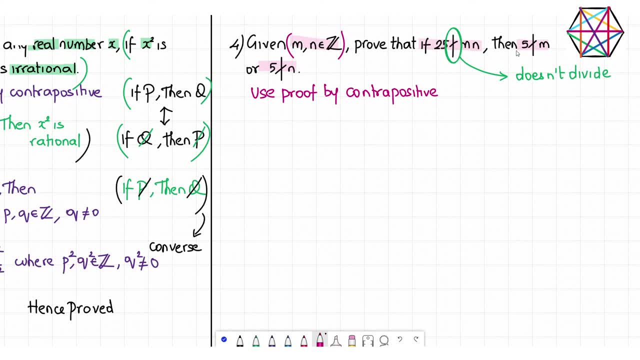 product of m and n. if 25 doesn't divide m n, then five divide. five doesn't divide m, or it's r okay, or five doesn't divide n. now i want you to come up with the contrapositive of this statement. contrapositive. i want you to come up with the contrapositive. 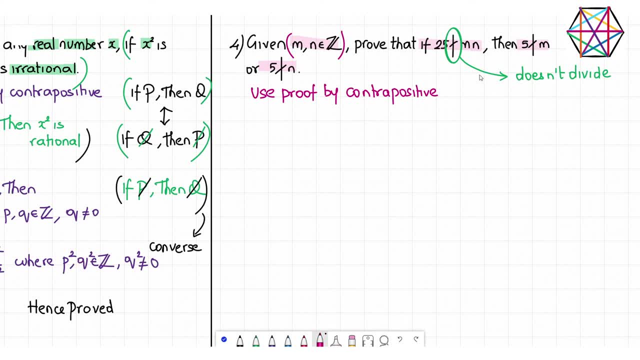 yeah, this is the original statement. this is the original statement. give me the contrapositive of it. yeah, once again you are giving me converse. you are giving me exactly this. listen that listen. that if part is called as p. that if part if some condition is there, that if 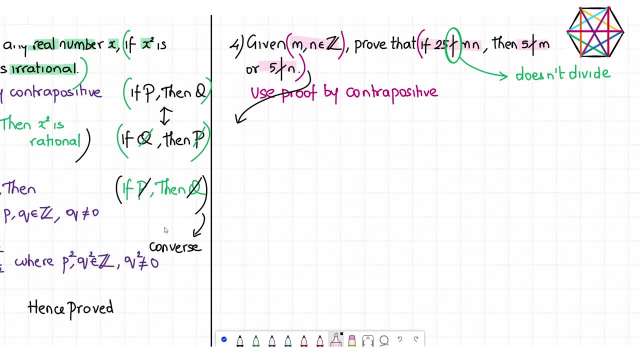 part is called as p and then part is q. right, if part we call it, we denote it by the letter p and then part p denoted by letter q. what you gave me is: if not p, then not q, that is exactly what you're giving me. that's totally wrong. what are you supposed to give me? if not q, then not p? yeah, 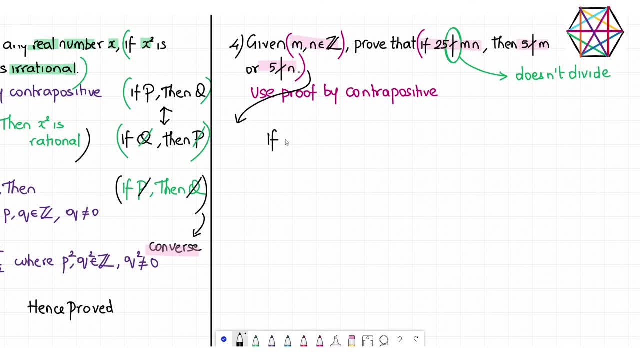 if not q, no, no, no, no, no, no. if five divides m and five divides n, you understand why? because it's not, we are negating it, we are negating it. okay, and here comes a very, very important thing: when you negate, or you know what is the meaning. 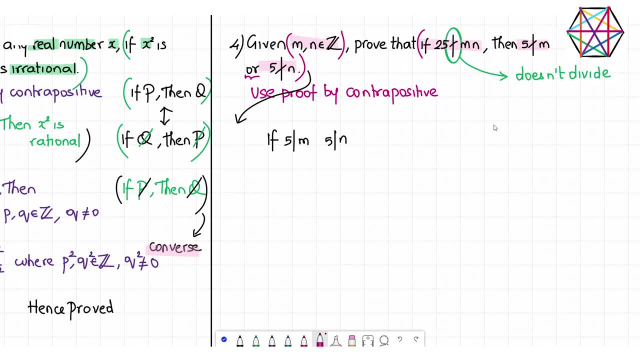 of it. you know what will happen. negate or what do you get. negate or we get. what do we get? and think about it. forget about mathematics, even in real life. that is what it means. that is how it works, even in real life. listen, think about it. okay, i will take just an example. i'm making up something. okay, i will take. 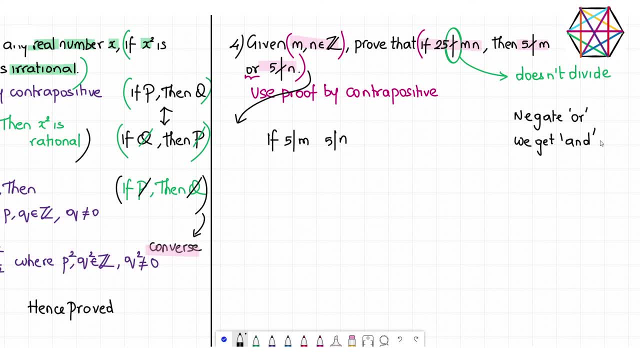 one extra class tomorrow or a day after. the negation is: i will not take extra class both tomorrow and day after, and day after yes or no, couldn't get it, or becoming, and yes or no, i'll take tea or coffee. the negation is i don't take tea and coffee. 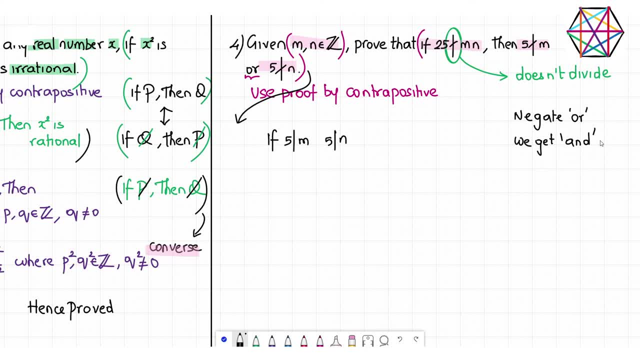 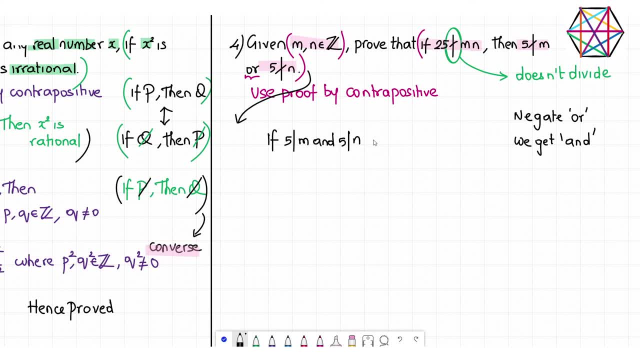 you get this and say that, okay, clearly, once again. okay, say it out loud: pi doesn't divide m, or five doesn't divide n, and the negation of that is: five divides n and or becomes and five divides n. right, and we're not done. then this is not q, what is not? b? 25 divides mmm. done, okay. so what is this? 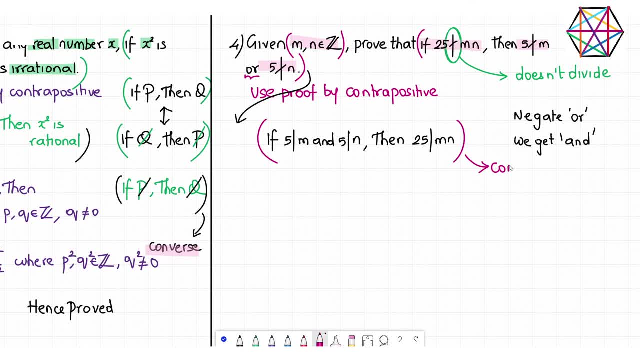 this is the contrapositive of the given statement. This is the contrapositive. So instead of proving the original statement, we are going to prove its contrapositive. Is that clear? Okay, now it is very easy to prove. Check this. Okay, check this. If 5 divides m and 5 divides n, it implies listen. 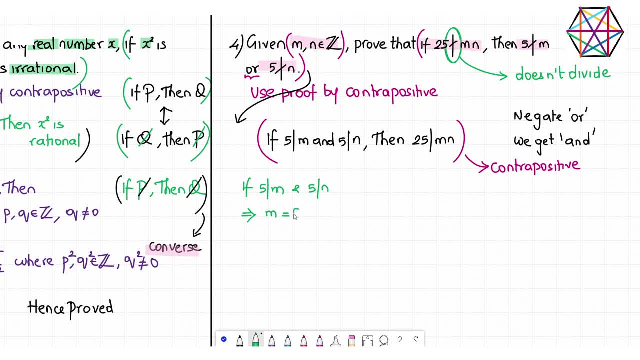 if 5 divides m, don't you see m is nothing but pi times p, where p is some integer Yes or no? If 5 divides m, m is nothing but a multiple of 5.. You see, you can say 3 divides 24, or you can say 24 is a multiple of 3, both the same. 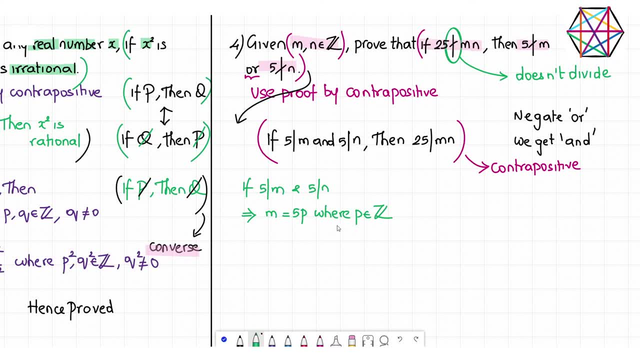 So 5 divides m. you can say that, or you can say m is a multiple of 5.. So m is a multiple of 5.. m is 5 times something. some integer p, I don't know what. it is Okay and.